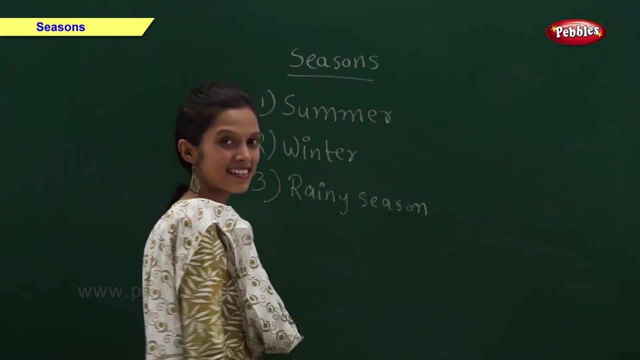 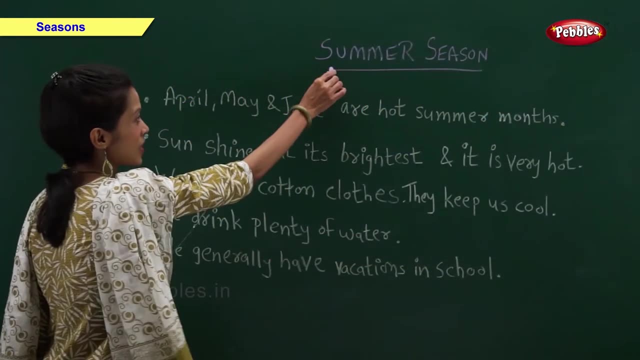 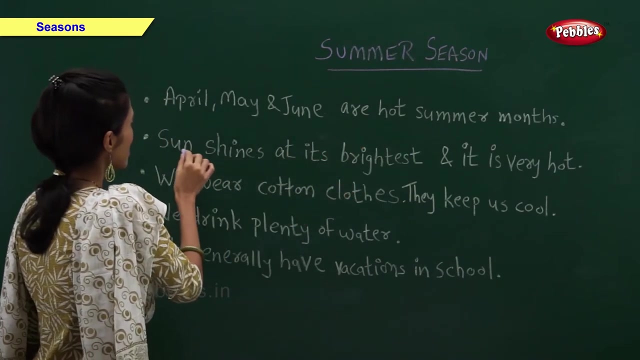 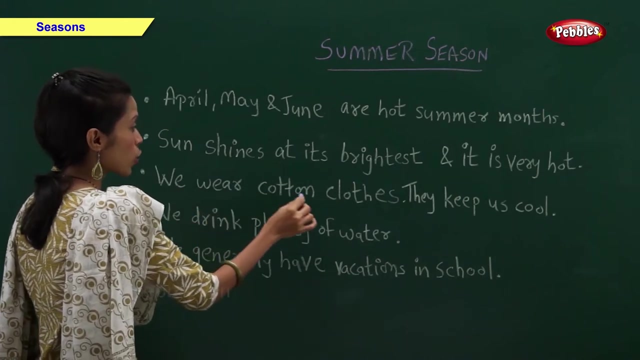 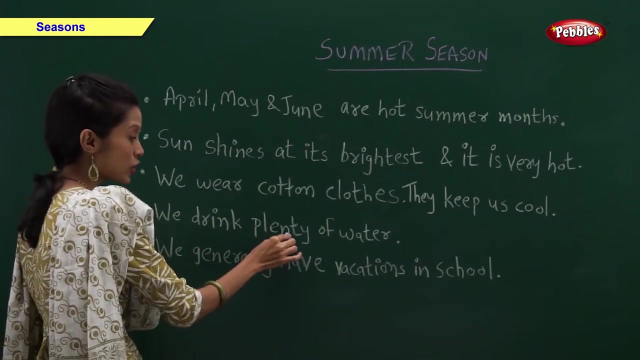 Now let us take a look at each season in detail. Summer season- April, May and June- are hot summer months. Sun shines at its brightest and it is very hot. We wear cotton clothes. Cotton clothes keep us cool. We drink plenty of water. 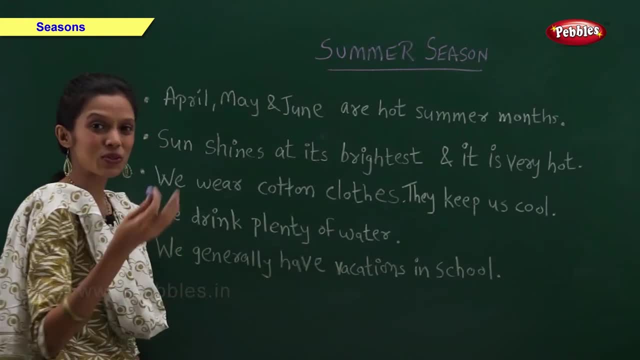 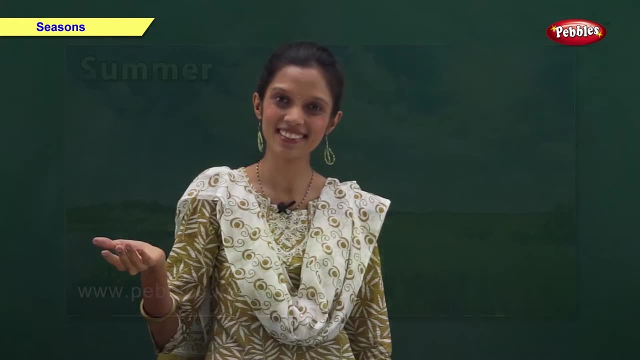 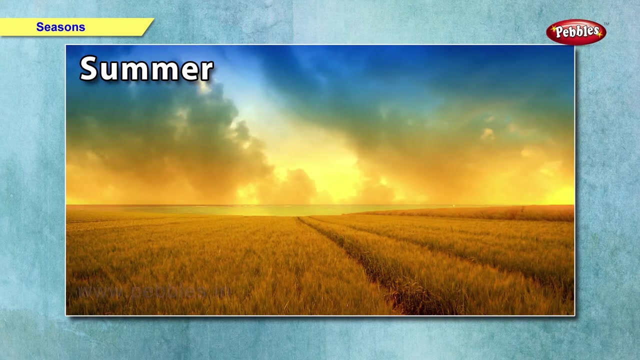 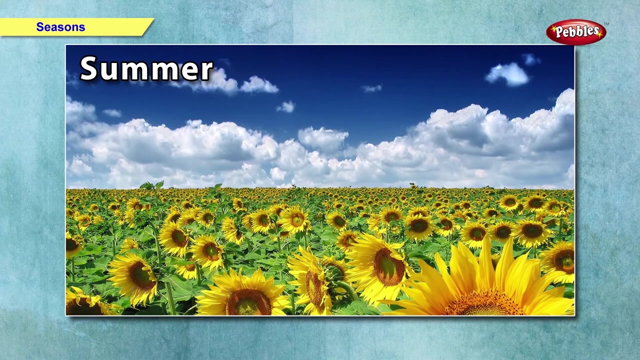 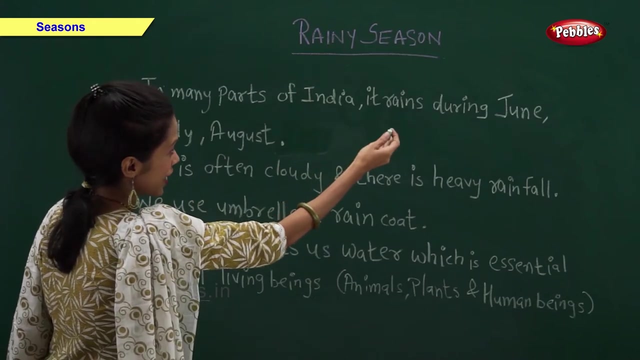 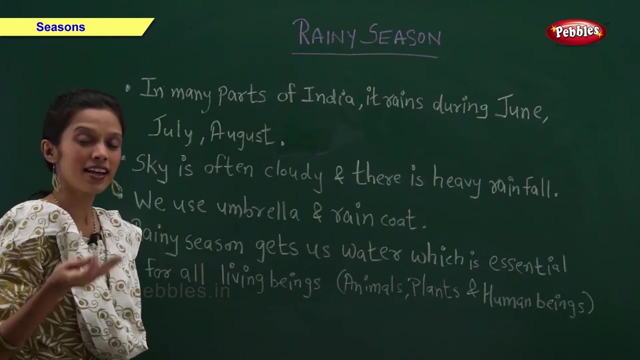 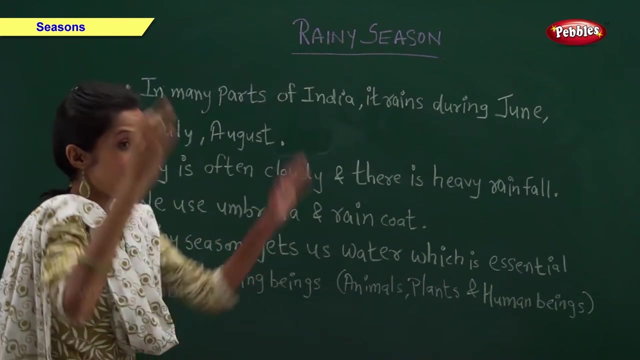 And generally we have vacations in school during summer season. Now I am going to show you some pictures of summer season Rainy season. In many parts of India it rains during June, July and August. Sometimes it also rains in September. Sky is often very cloudy and there is a heavy rainfall. 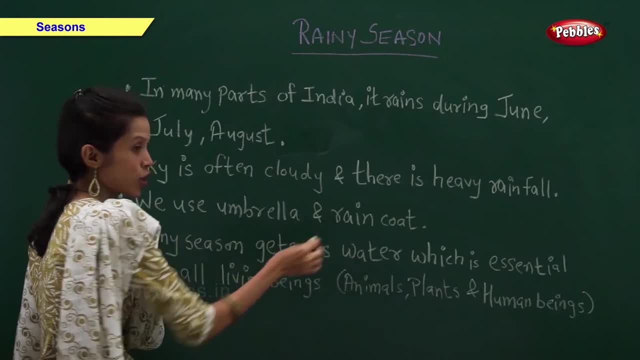 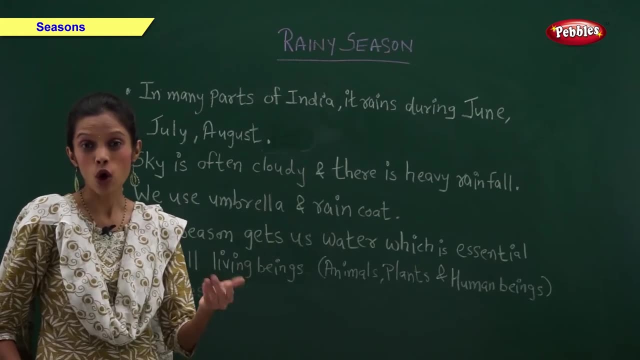 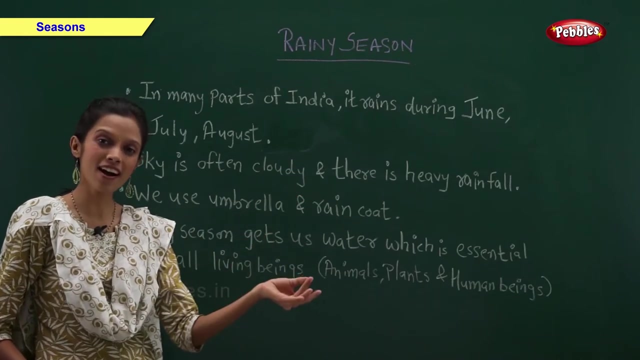 We use umbrella and raincoat. We use umbrella and raincoat To protect ourselves from getting wet. Rainy season gets us water, which is very essential for all of us, Like animals, human beings and plants. Now I am going to show you some pictures of rainy season. 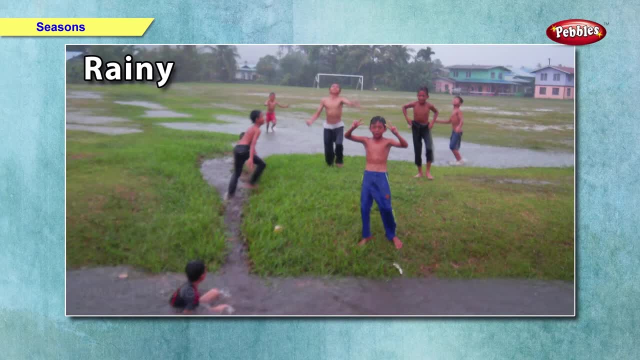 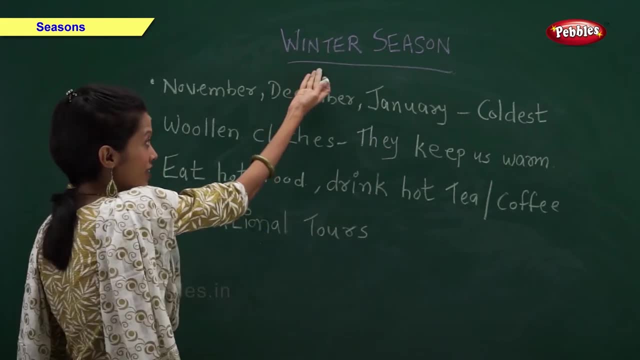 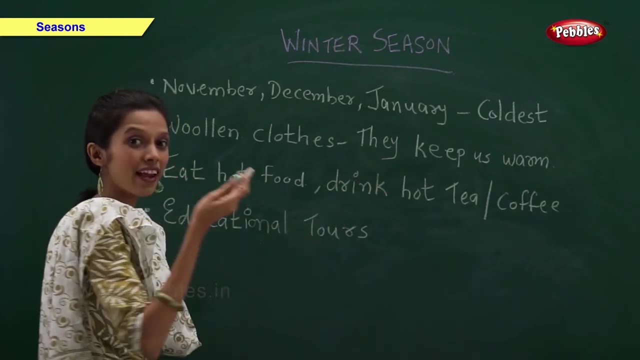 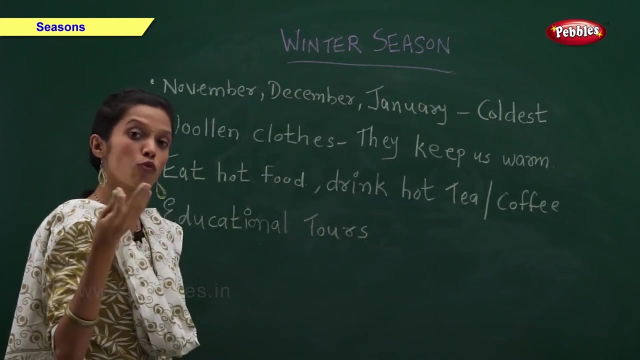 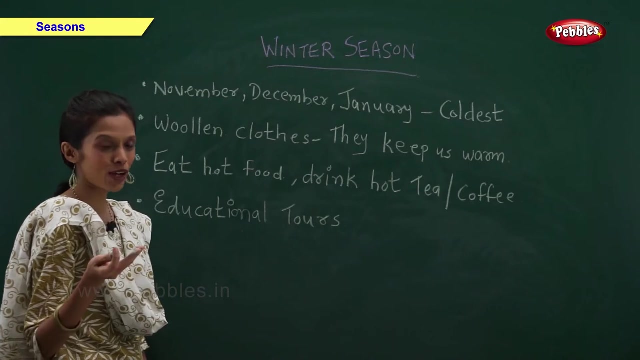 Winter season. It is very cold during winter season. November, December and January are coldest months. in India, We wear woolen clothes during winter season. They keep us warm. We generally like to eat hot food. during winter season. We also like to drink hot tea or coffee. 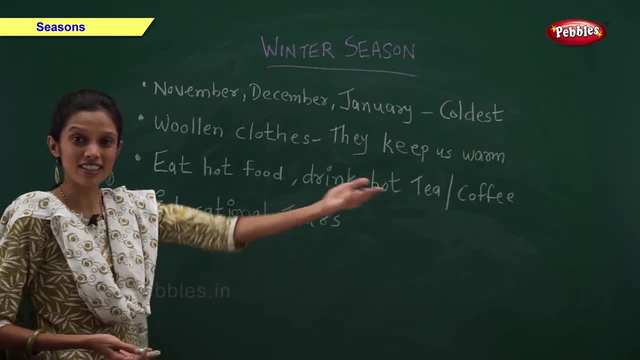 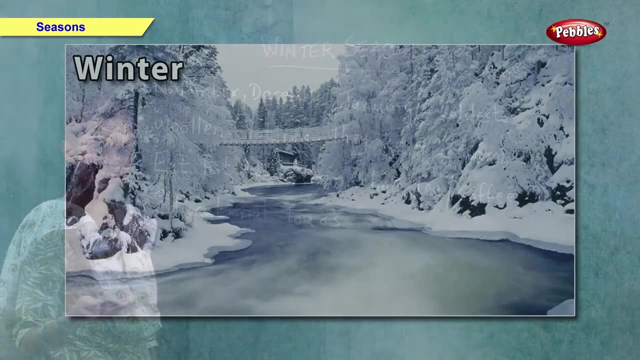 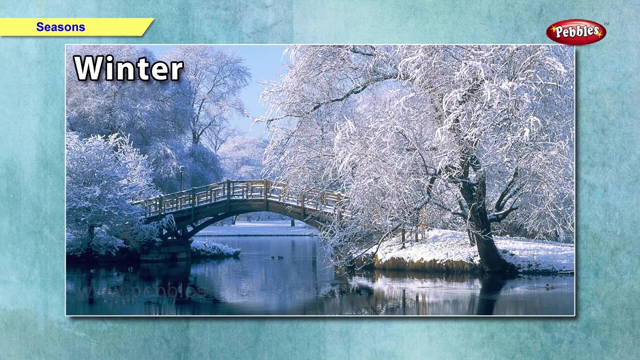 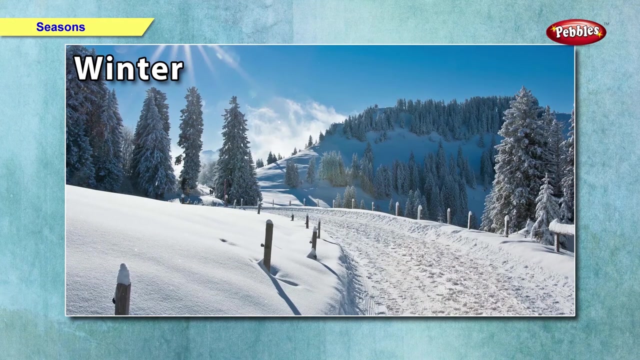 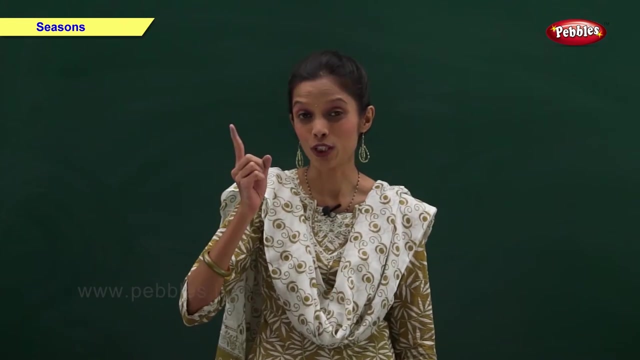 Winter is very good season for conducting tours, And many educational tours are conducted during winter season. There are two main seasons in India: Summer, rainy season and winter. The climate is different in all three different seasons. It is very hot in summer season. 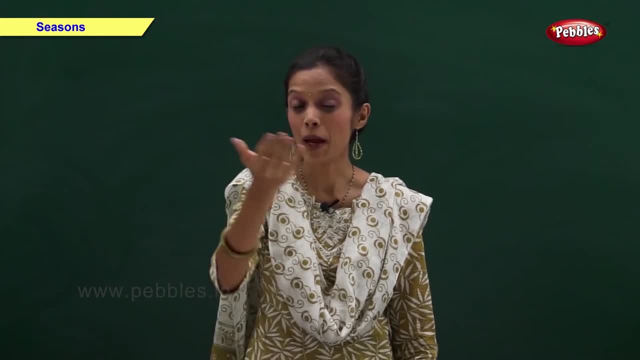 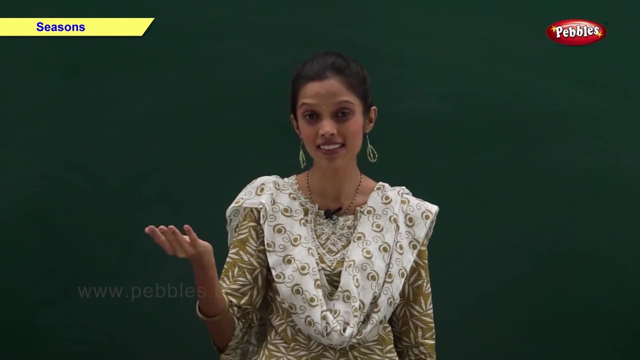 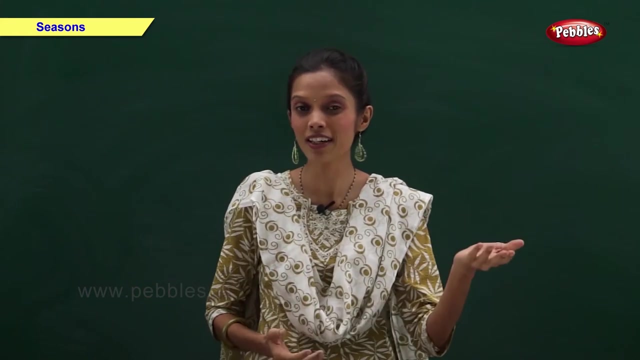 It rains in rainy season And it is very cold in winter season. It is very hot in summer season. There are three main seasons in India: Summer, rainy season and winter. And it is very cold in winter. We wear different kind of clothes in different seasons. 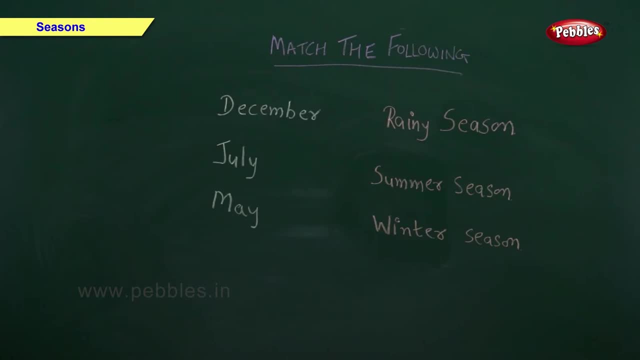 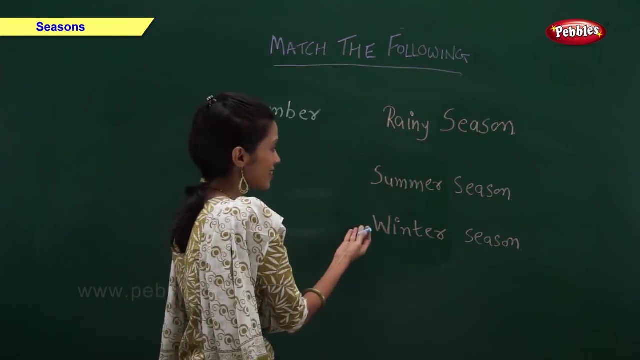 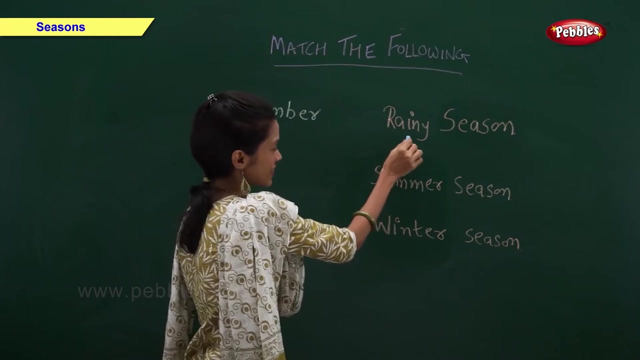 Match the following: On one side I have written the months and other side I have written the seasons. You have to match them. December, Month of December falls. in which season Do it falls? in summer season, No. Which other season? Rainy season, No. 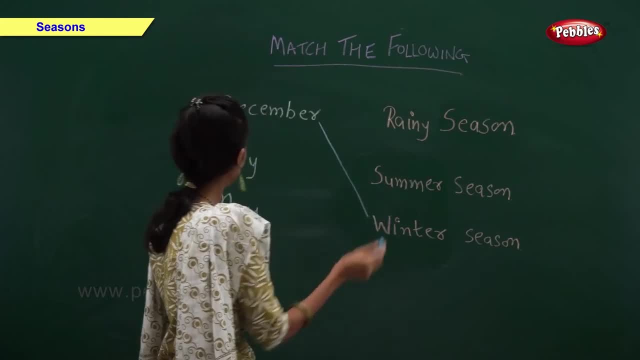 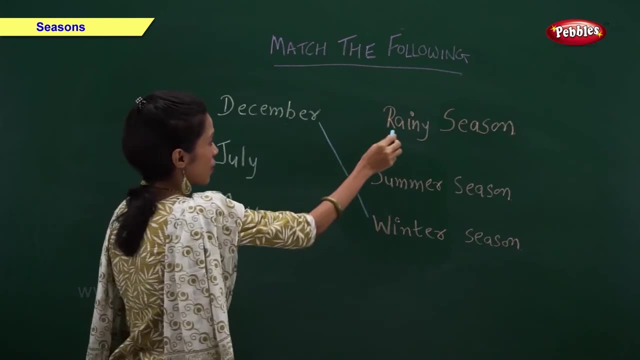 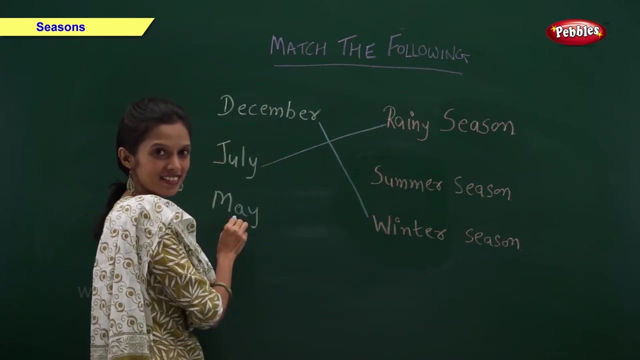 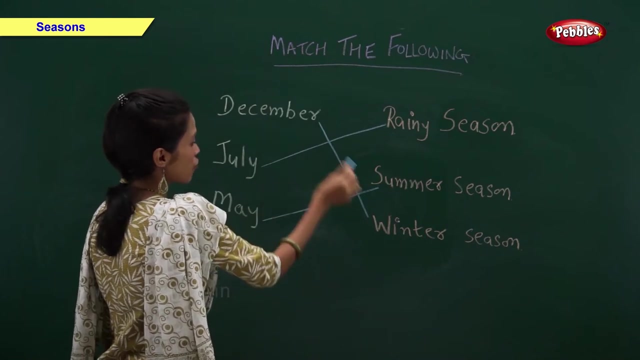 Yes, it falls in winter season, July. Month of July falls in which season? Rainy season: Yes. Next month of May falls in which season? Yes, summer season. So December falls in winter season. July falls in rainy season. 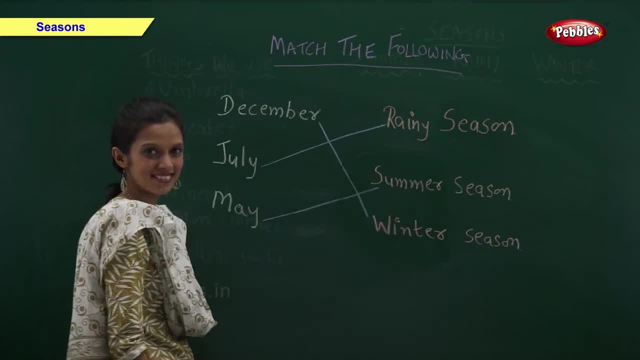 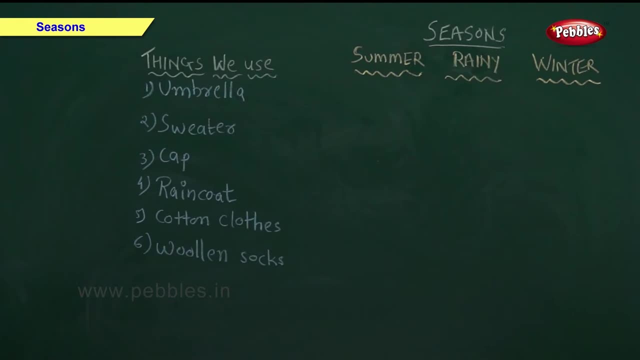 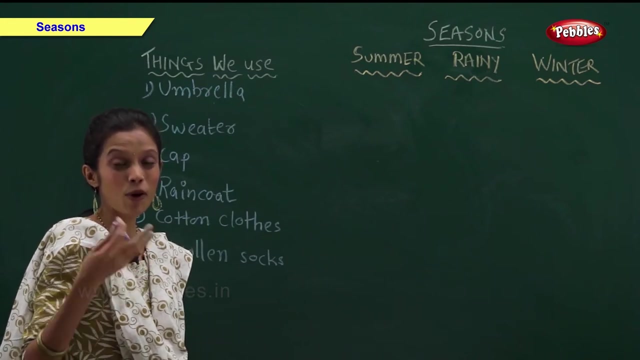 And May falls in summer season. I have written a list of things we use. You have to put them under correct season. You have to put them under correct season Umbrella: In which season do we use umbrella? Come on fast, I told you earlier. 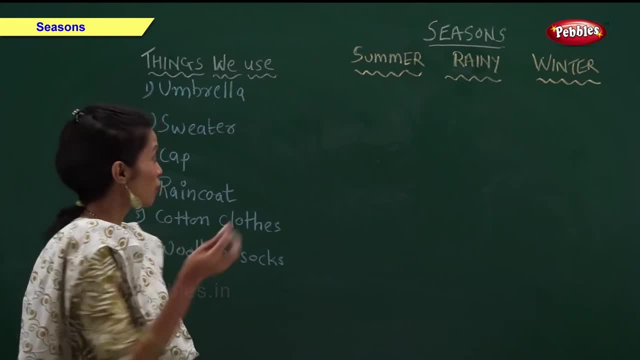 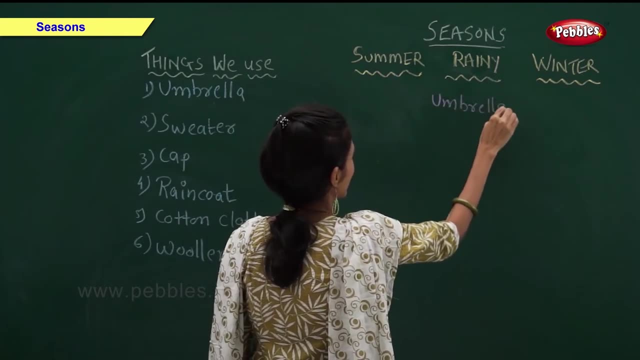 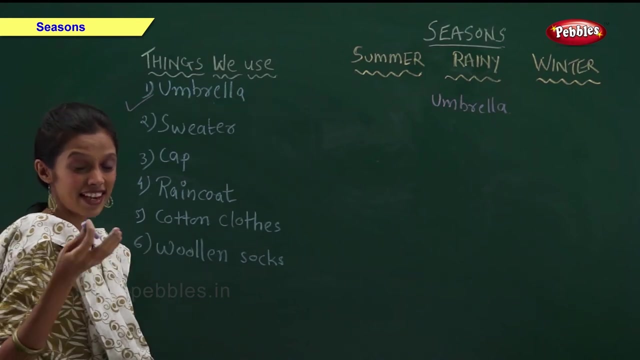 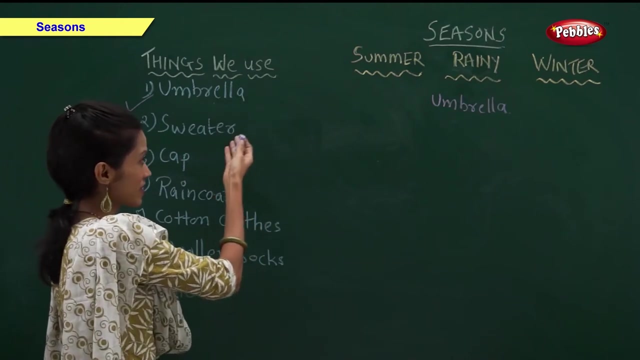 Do we use umbrella in summer? No, We use umbrella in rainy season. Rainy season, In which season do we use umbrella? Do we use sweater? Yes, tell me. In rainy season. do we use sweater? No, We use sweater in winter. 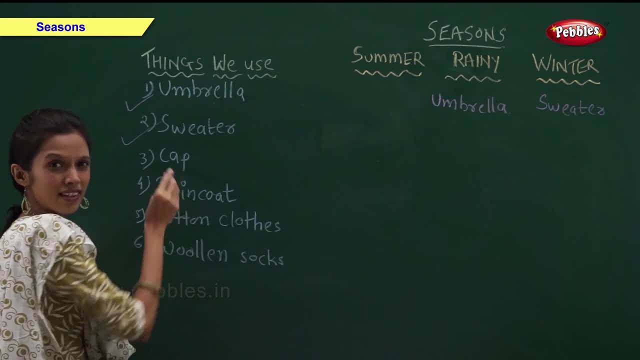 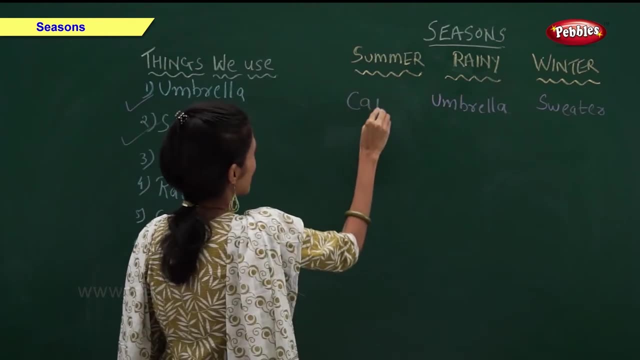 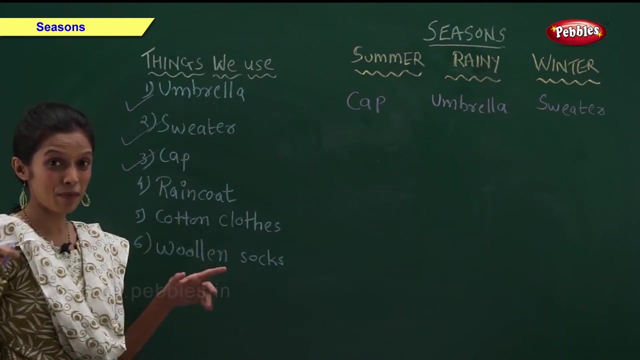 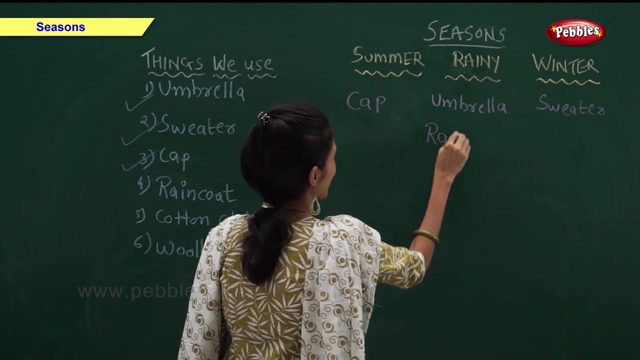 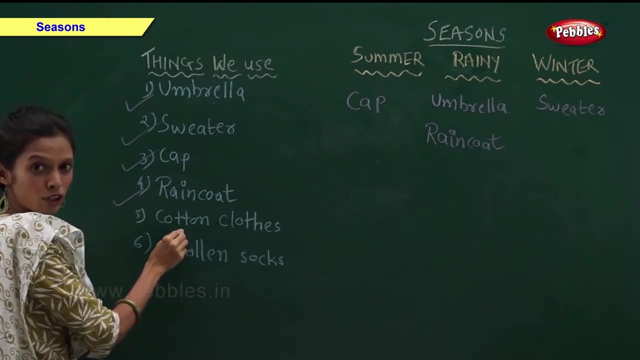 In which season do we use cap? Yes, fast, Yes, in summer we use cap. In which season do we use raincoat? In which season do we use raincoat? Remember, Yes, we use raincoat in rainy season. When do we use cotton clothes? 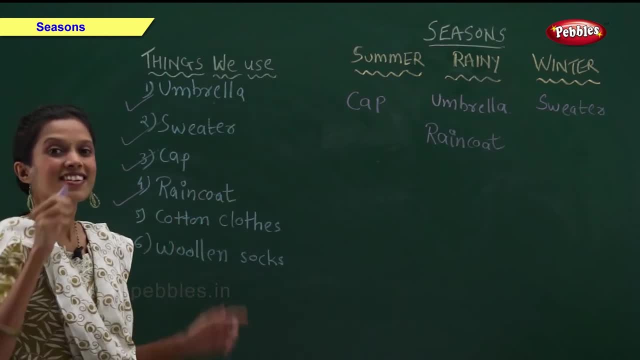 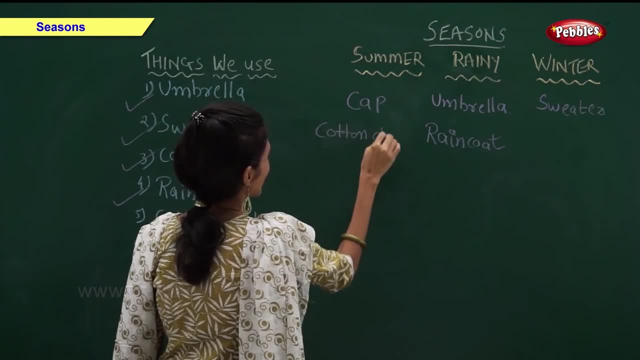 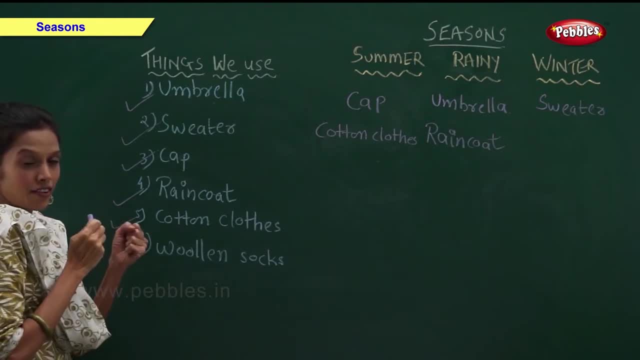 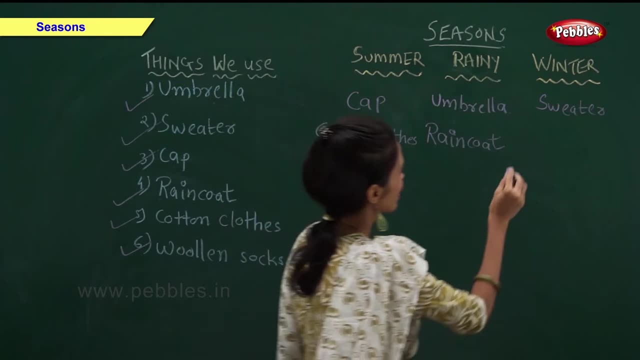 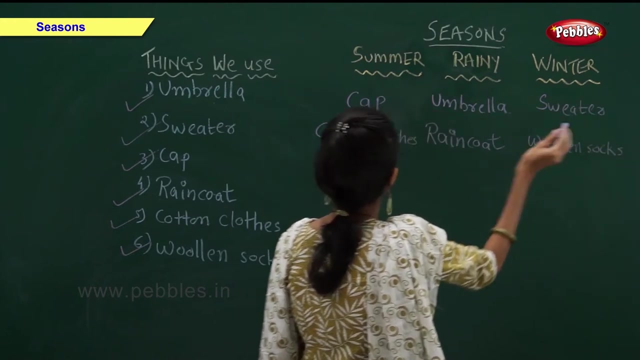 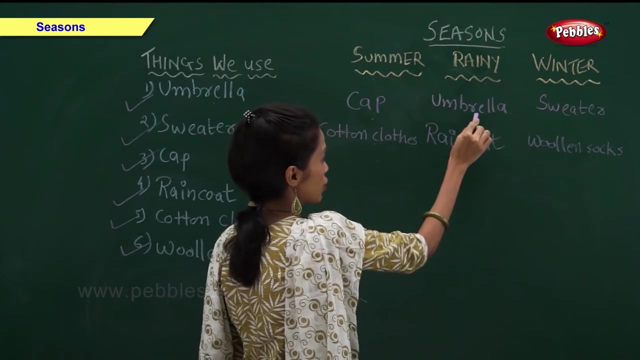 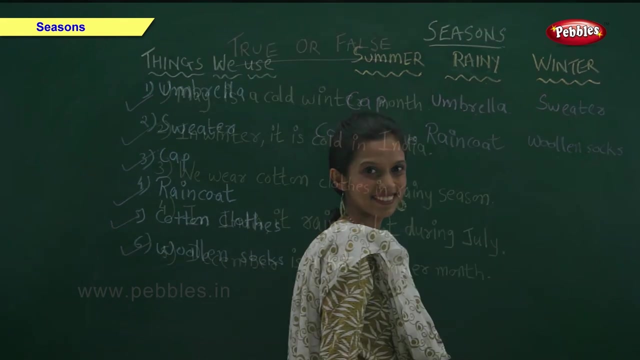 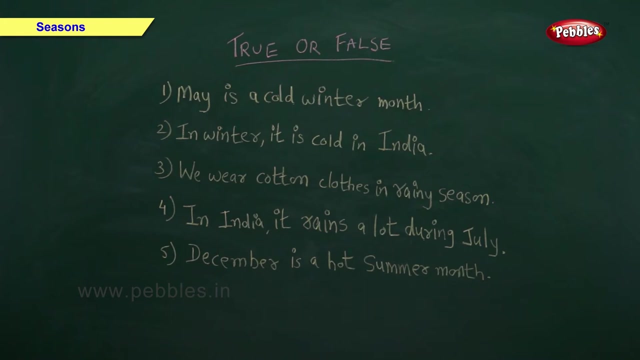 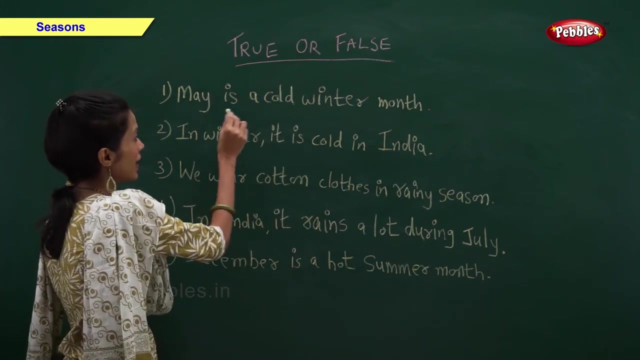 When we use woolen socks. Remember, Yes, in winter we use woolen socks. So in summer we use cap and cotton in clothes, In rainy season we use umbrella and raincoat, And in winter we use sweater and woolen socks. True or false? True or false? May is a cold winter month. True or false? 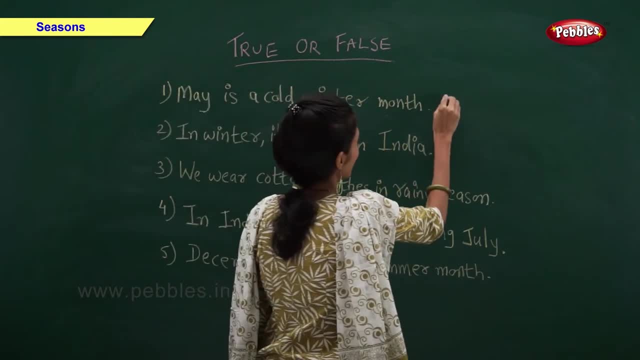 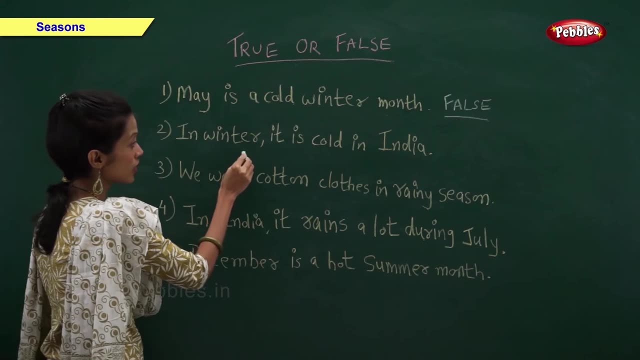 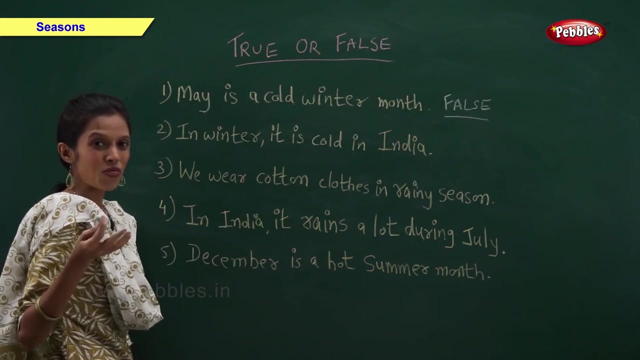 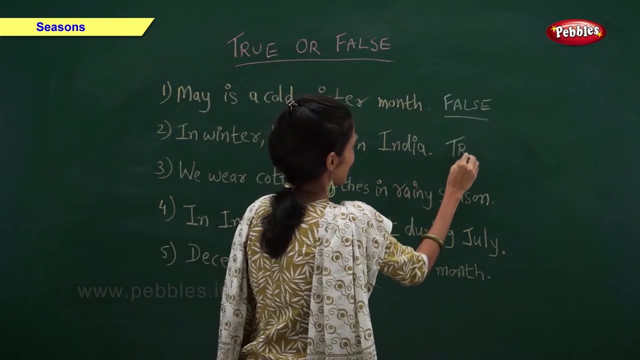 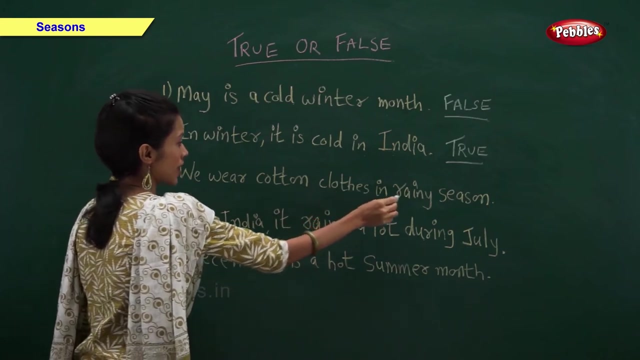 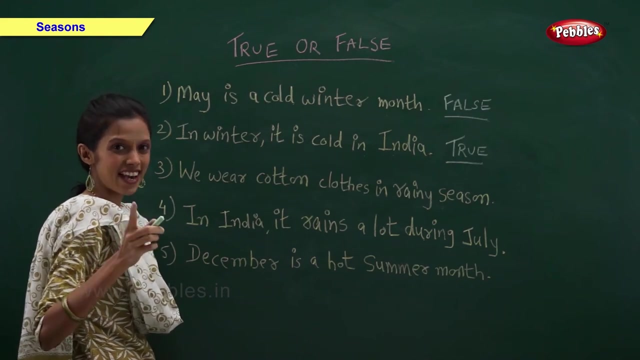 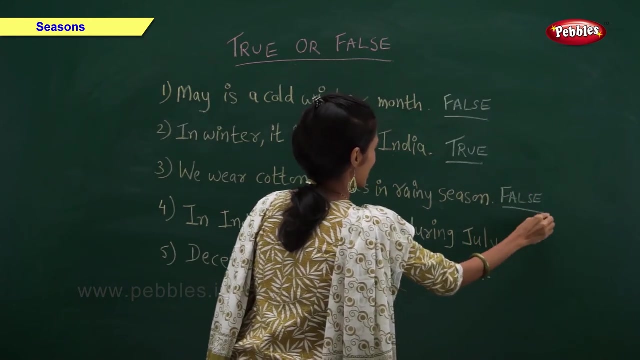 Yes, false. In winter it is cold in India. True or false? False, No, True. in winter it is cold. in India, We wear cotton clothes in rainy season. Is it true or false? Come on fast. Yes, false In India. 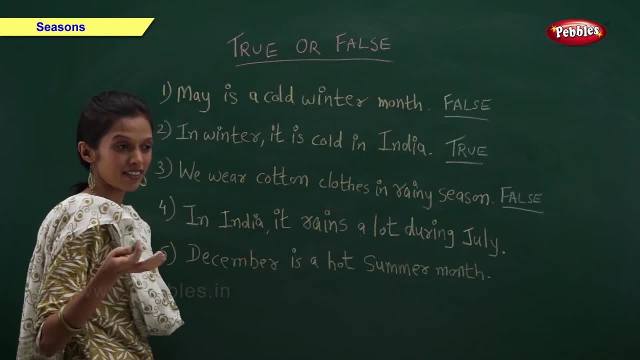 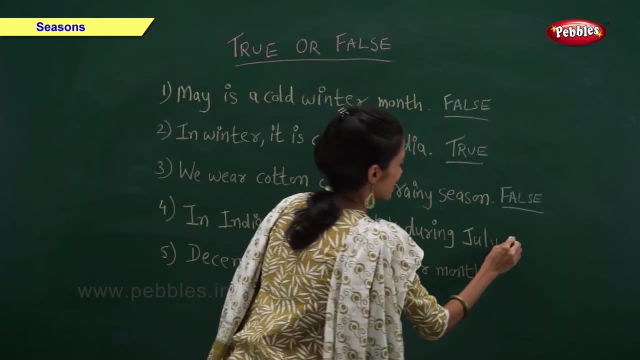 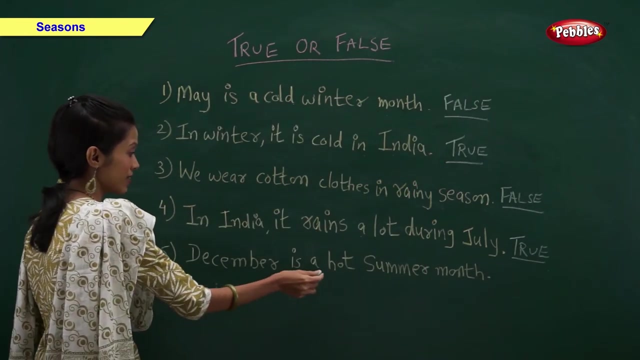 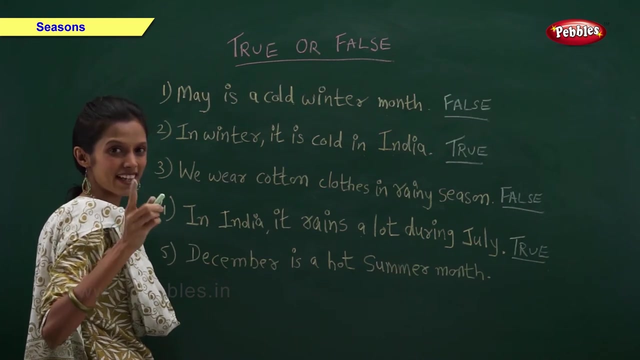 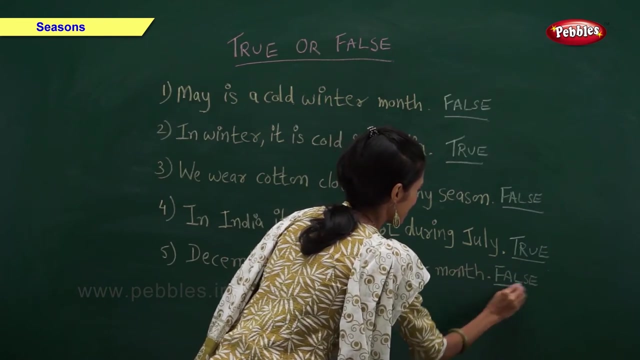 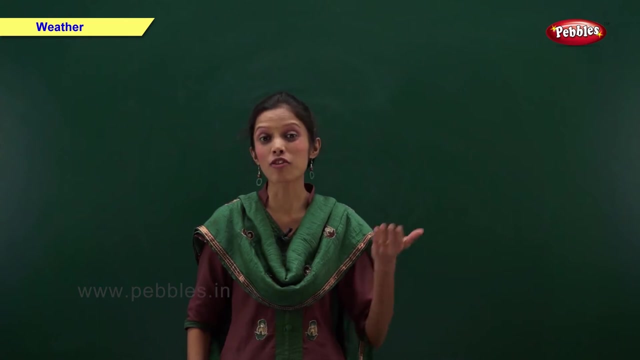 it rains a lot during July. Remember the months I told earlier? Yes, true, December is a hot summer month. True or false? Come on fast. Yes, false, Weather is a climatic condition on the earth. Weather affects the way we live our life. Sun. 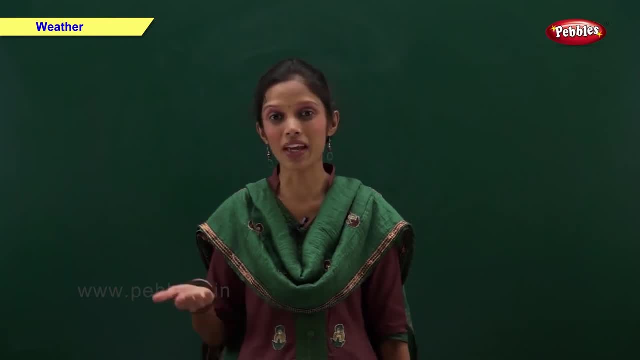 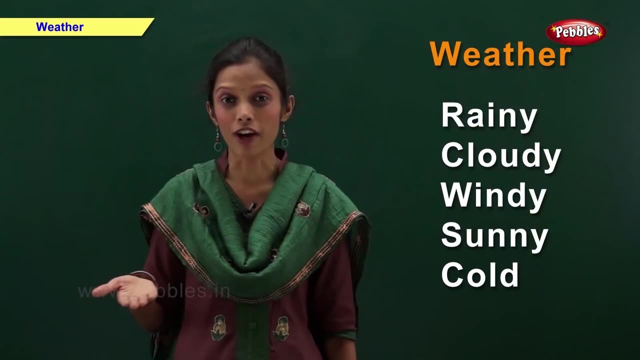 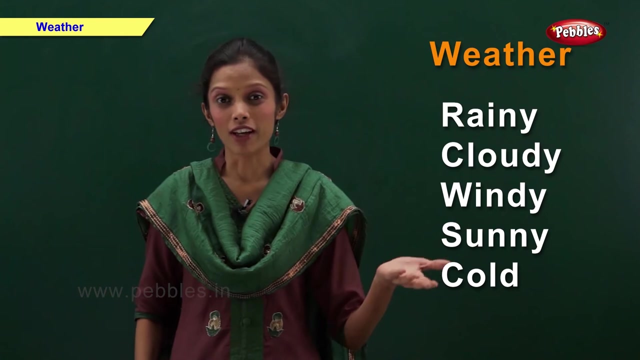 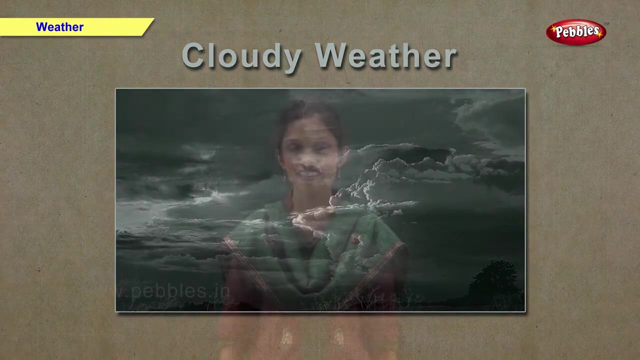 shine. rain and wind on a day makes the weather. Weather can be rainy, cloudy, windy, sunny or cold. Weather keeps on changing. The conditions of air are called as weather. Sometimes weather is a cold weather. Sometimes weather is a cold weather. Sometimes weather is a cold weather. 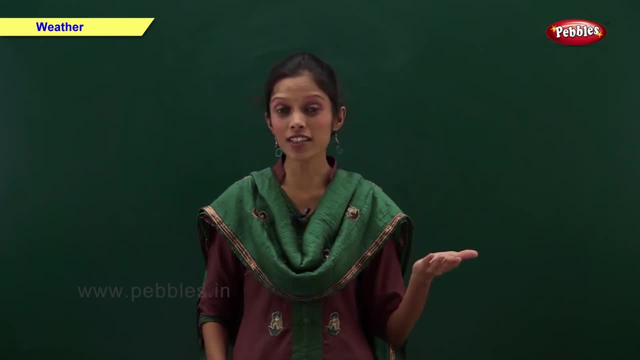 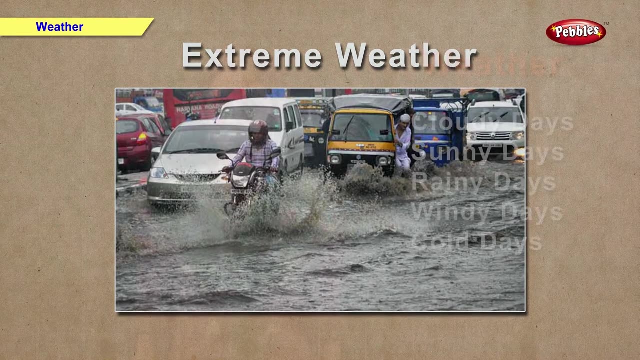 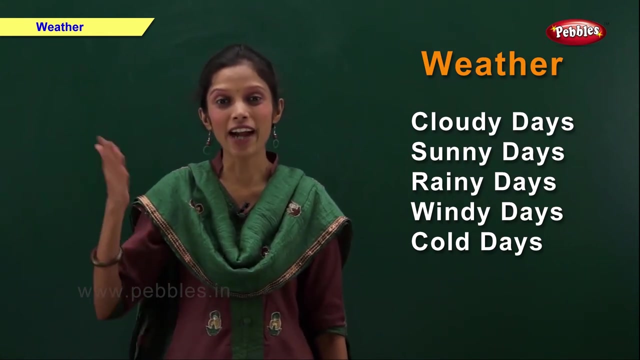 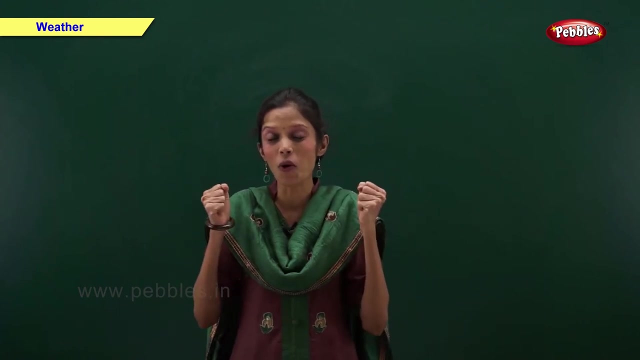 Weather can be to its extreme. Weather really affects the way we live our life. We have cloudy days, sunny days, rainy days, windy days and cold days. All these are different climatic conditions. On the hills weather is cold and on the plains weather is hot. 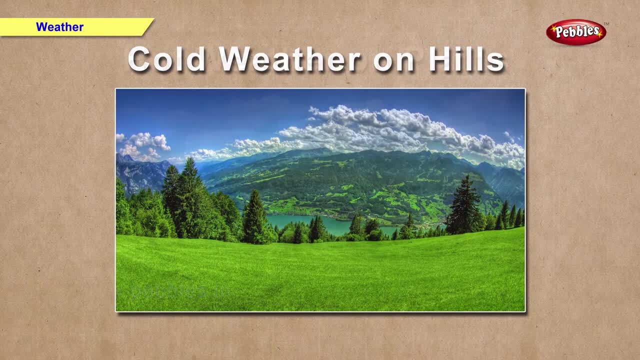 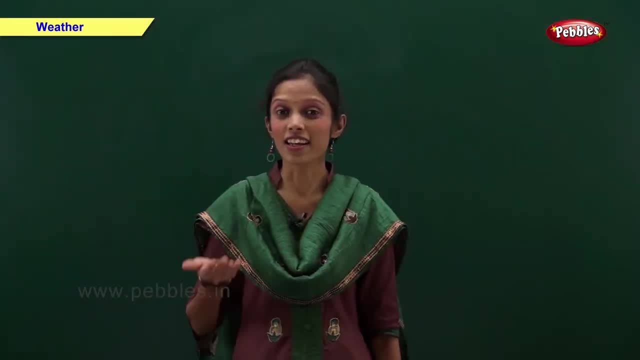 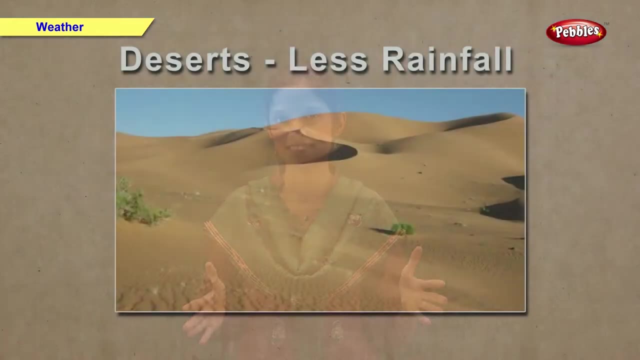 There can be several Amanda County claustrophobics in places with heavy rainfall. Moreover, during winter, select erhaltenwaters that can be claimed as the kind that come on down in the ice or at pouring coming from the lake. All different organizations around. 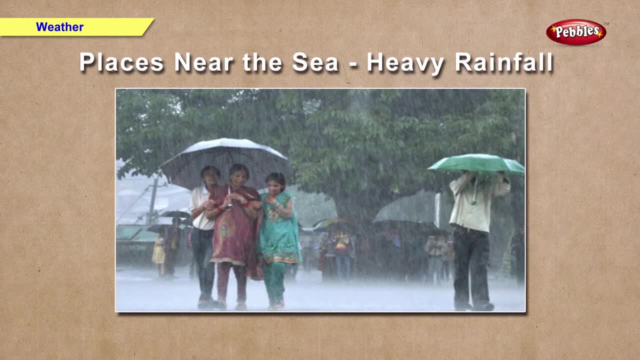 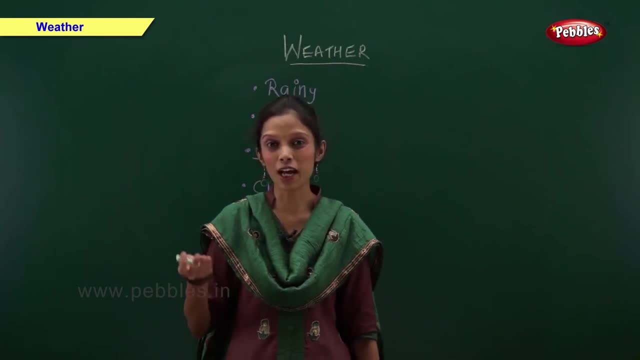 the world have different flow patterns, like shadow, каким you can't tell. we say: if you want to do what's called, follow Google Drive June 1st September. well known for its different climatic conditions, Different climatic conditions of India are as follows: 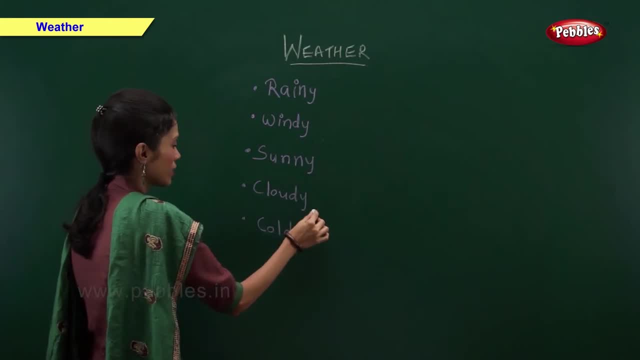 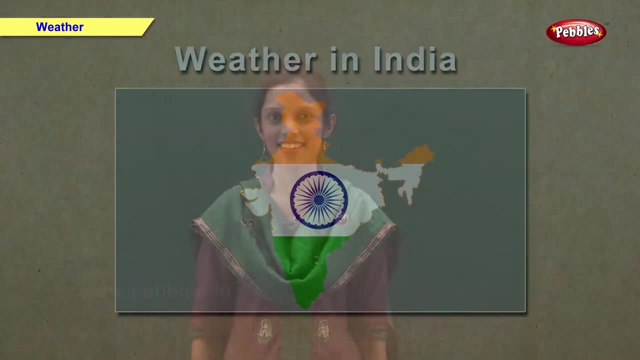 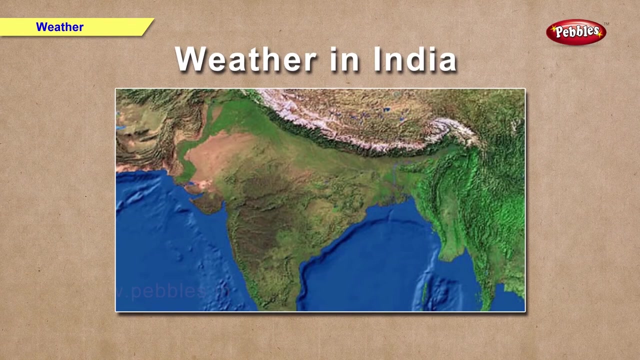 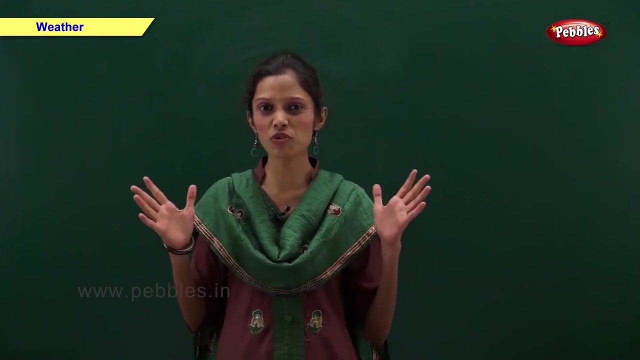 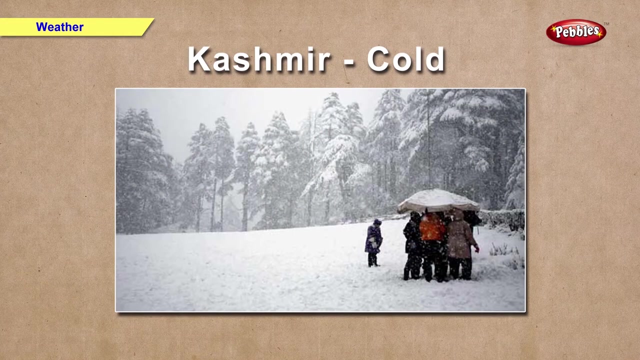 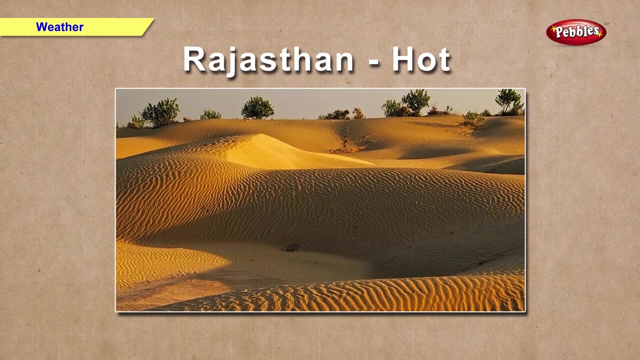 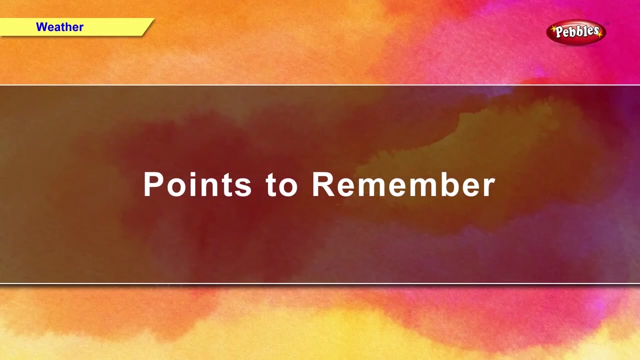 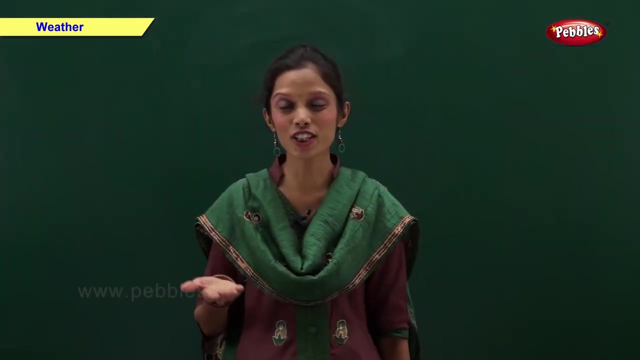 Rainy, windy, sunny, cloudy and cold conditions. Different places in India have different weather. In Kashmir it is very cold, In Rajasthan it is very hot And in Mumbai we have heavy rainfall. Points to remember Conditions of air is called weather. 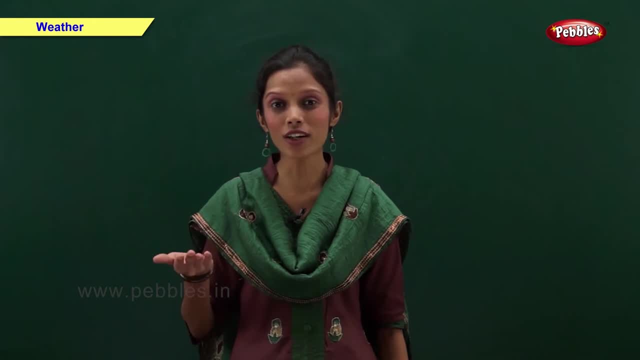 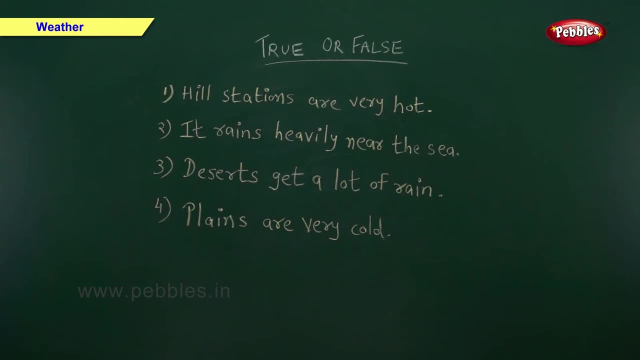 Hill stations are cold, Plains are hot And it rains heavily near sea. True or False? Hill stations are wet, Very hot, True or False? Come on tell me: Yes, False. It rains heavily near the sea. True or False? 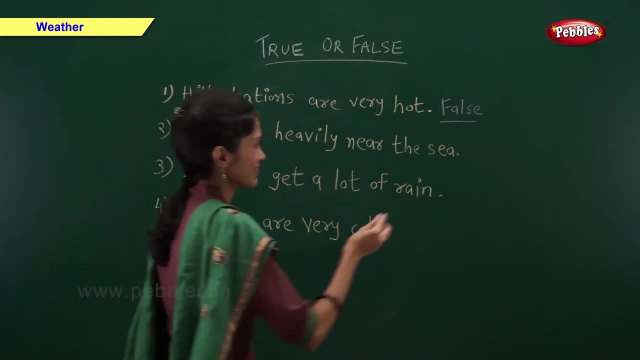 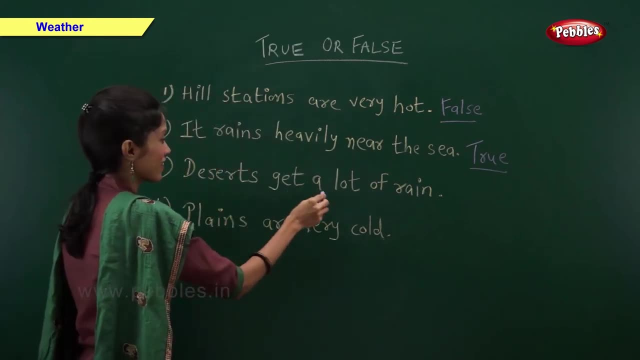 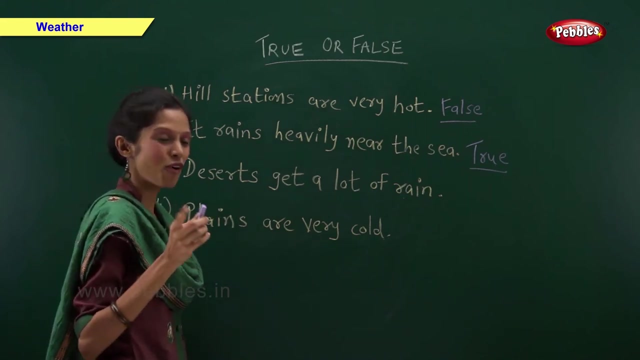 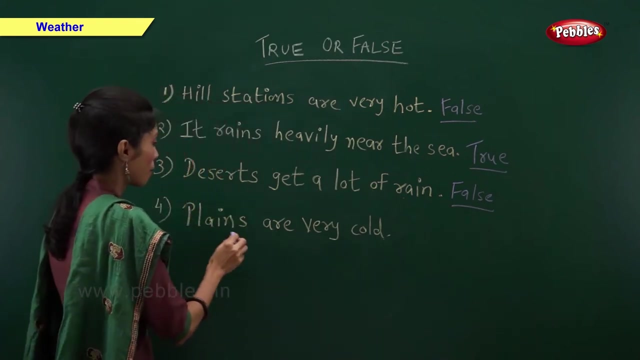 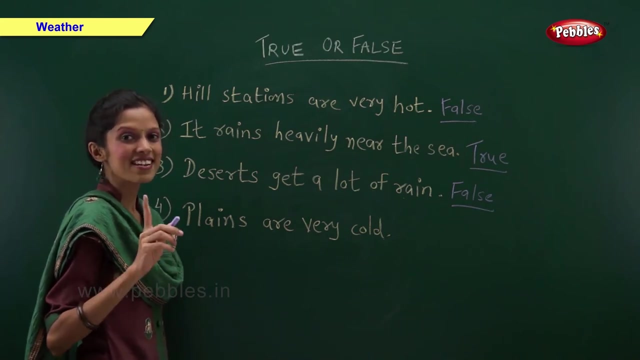 Come on fast. Yes, True, Deserts get a lot of rain. True or False? I told you earlier: Yes, False Plains are very cold. True or False? Come on fast, tell me. Yes, False, Match the Column. 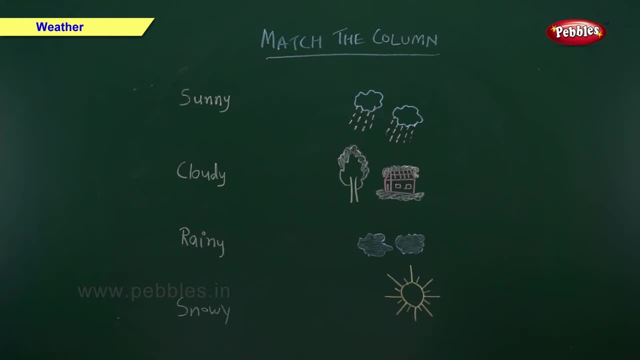 On one side I have written the different weathers and on the other side there are pictures. You have to match them. You have to match the Column Sunny. Which picture do you think represents the sunny weather? This, this, this or this? 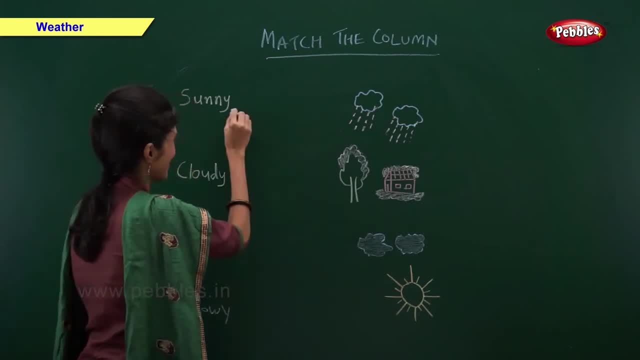 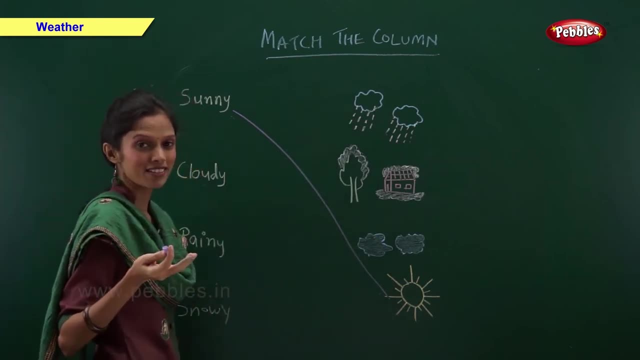 Come on tell me: Yes, this one Cloudy Which picture out of these represents the sunny weather. which picture out of these represents the cloudy weather, This, this or this? Yes, this one Rainy Which picture out of these two represents the rainy condition. 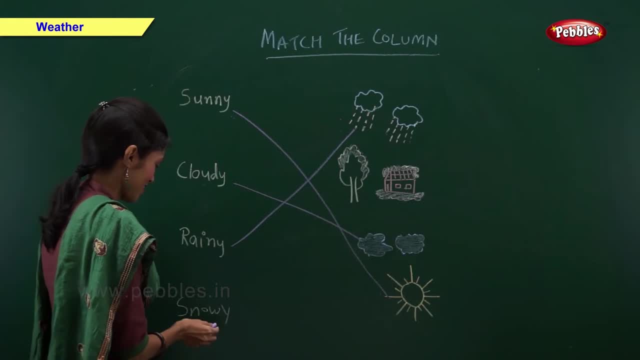 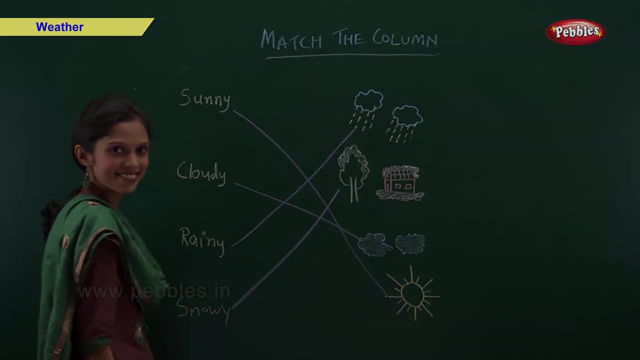 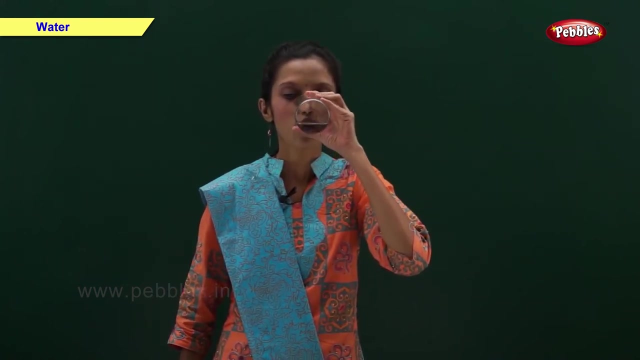 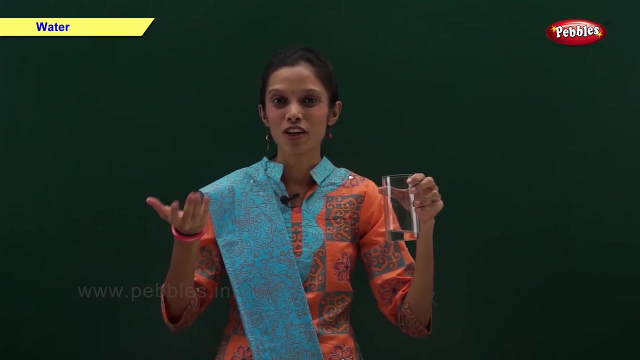 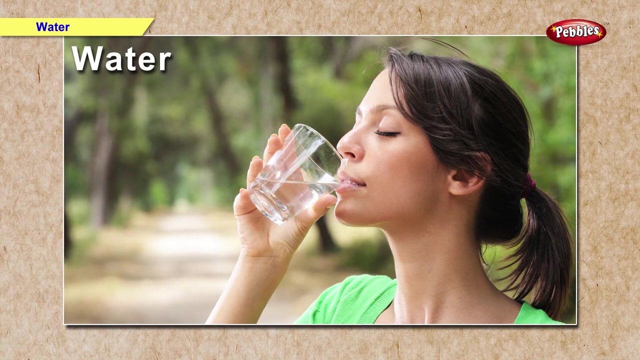 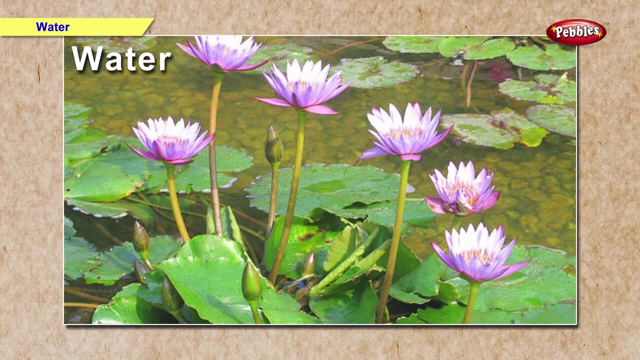 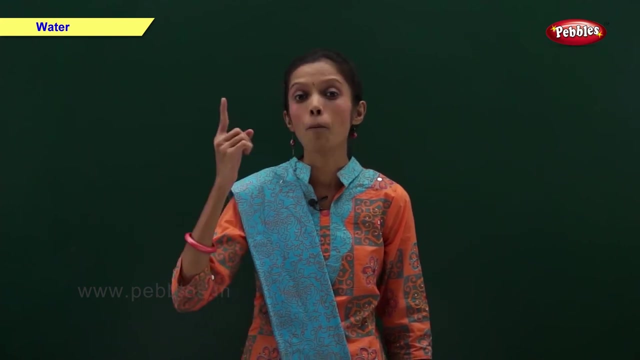 Yes, this one Snowy, This picture represents the snowy weather. So, friends, do you know what we are going to learn today? Yes, today we are going to learn about water. Water is very important to us. Men, animals and plants cannot live without water. 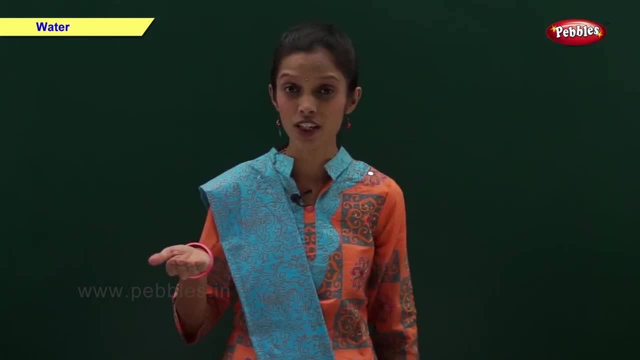 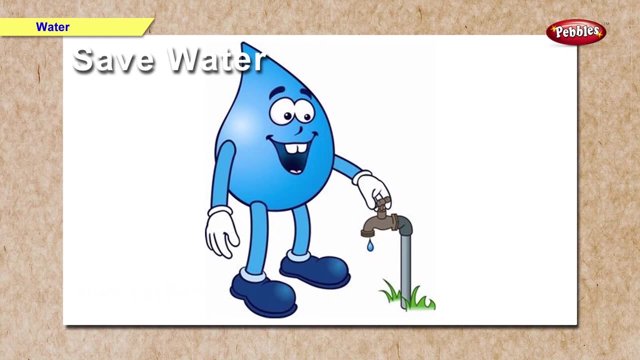 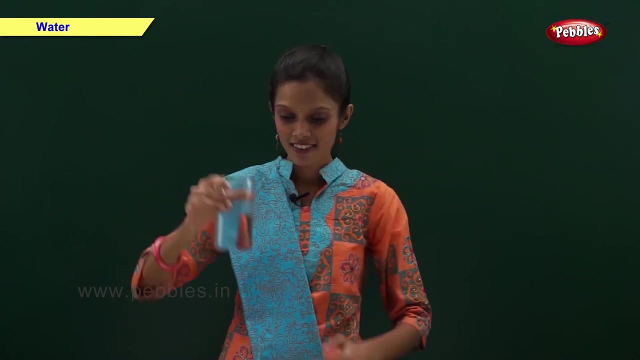 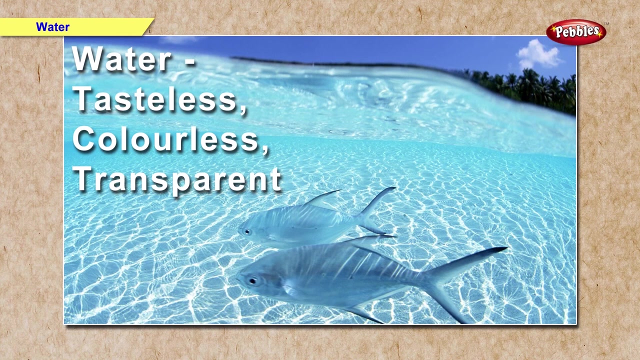 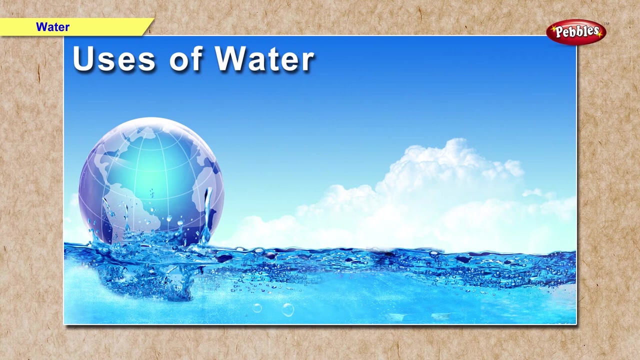 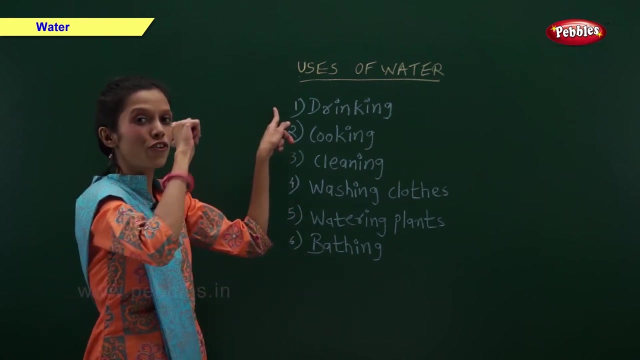 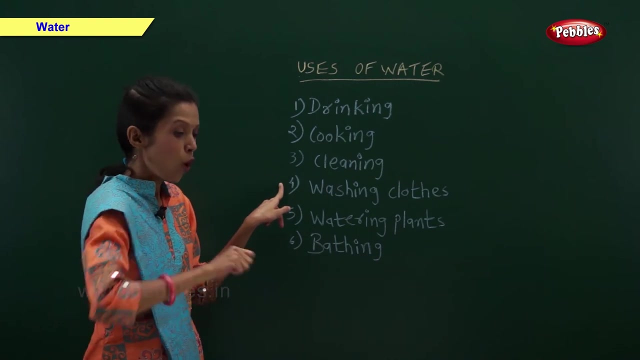 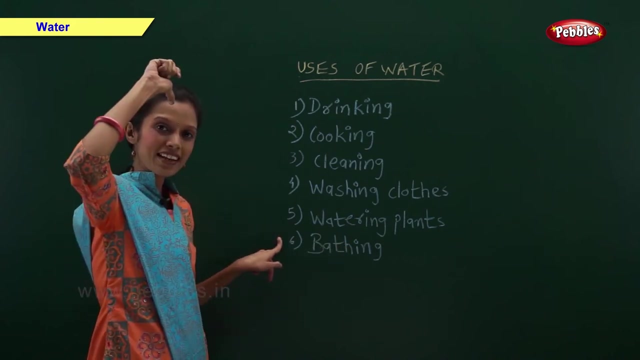 Everyone needs water. Water is very precious and we should not waste it. Water is tasteless, colourless and transparent. Uses of water. Uses of water: We use water. We use water for drinking, cooking, cleaning washing clothes, watering plants and bathing. 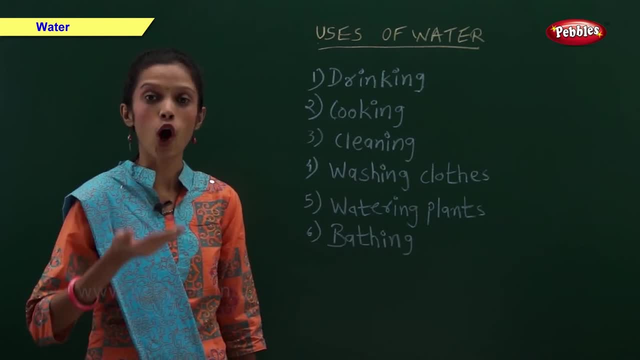 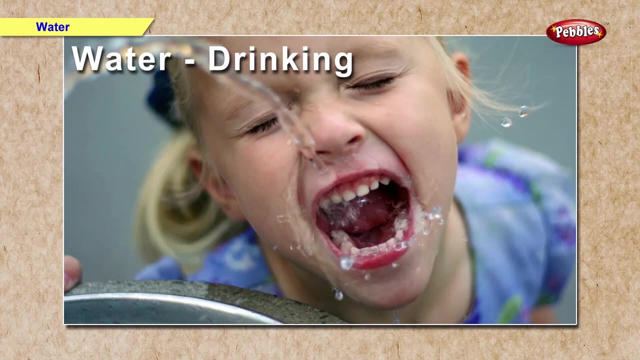 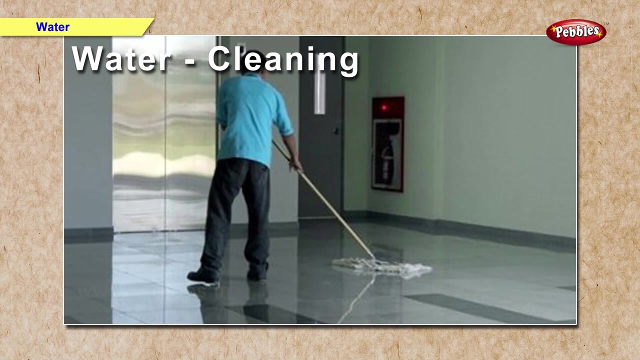 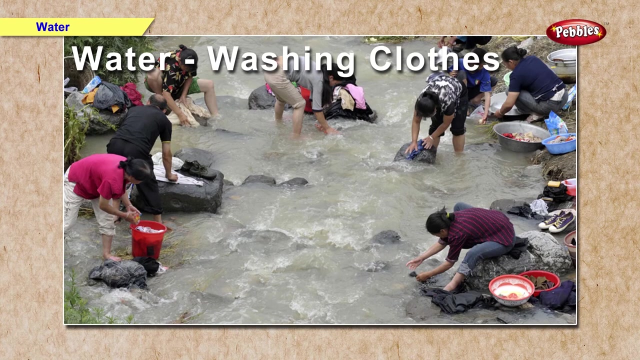 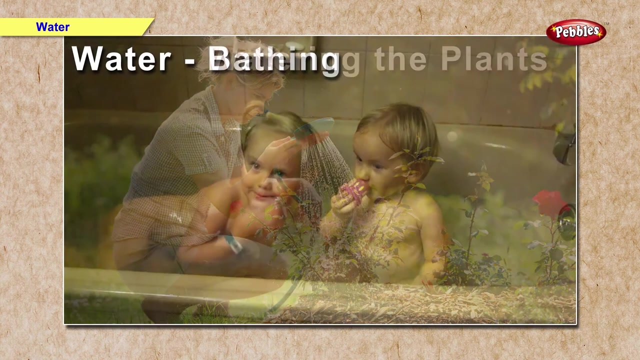 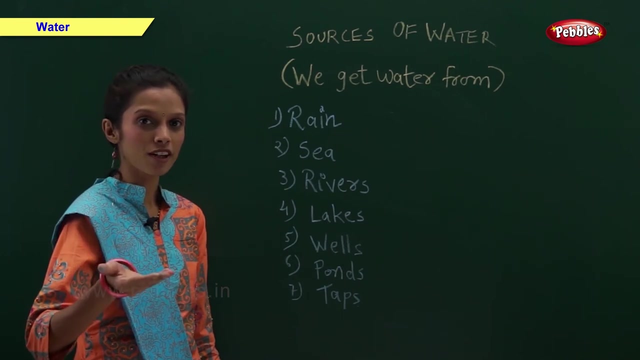 Now, friends, I will show you some pictures of various uses of water Drinking. We use water for drinking, cooking, cleaning, washing clothes, watering plants and bathing. Sources of water. Sources of water, That is, We get water from. We get water from. 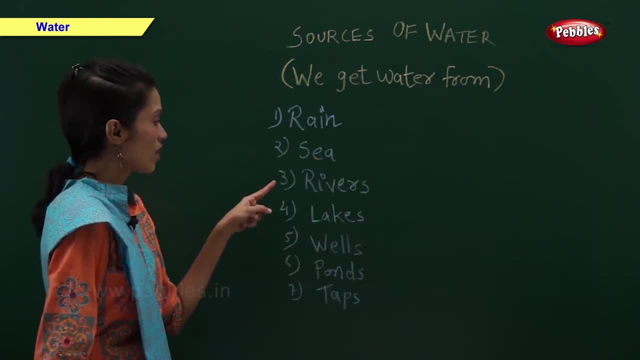 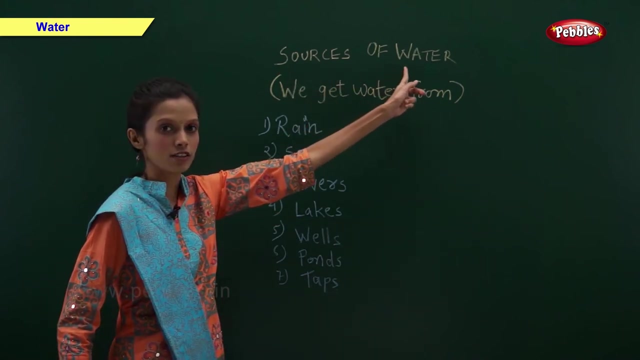 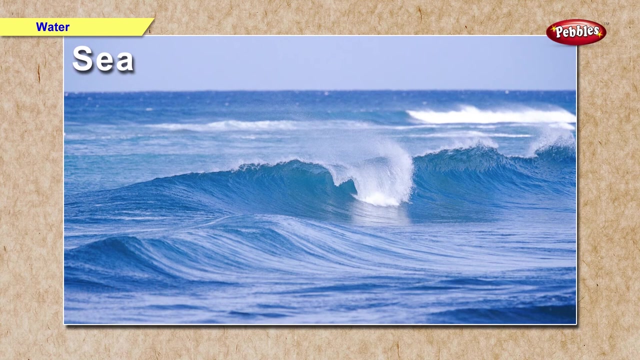 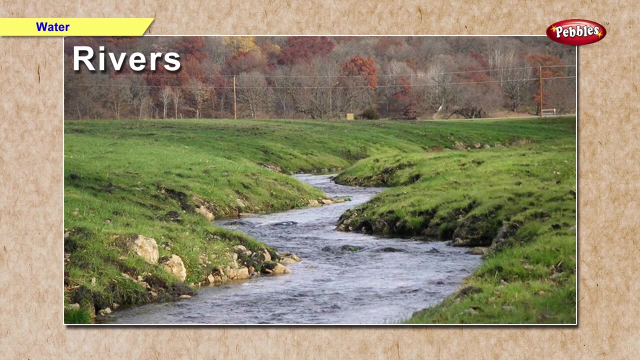 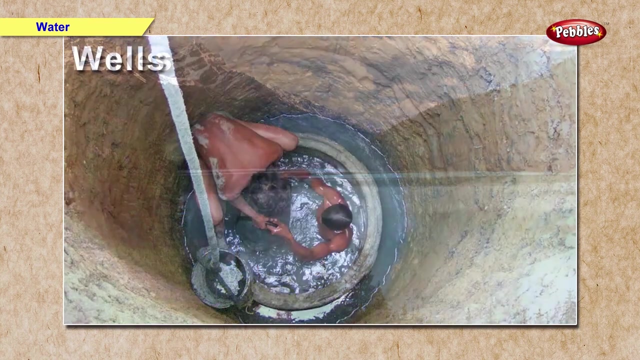 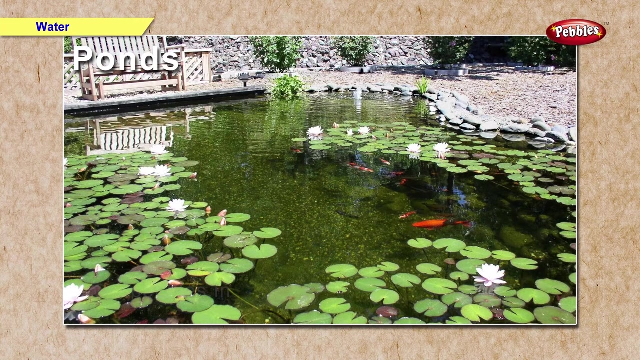 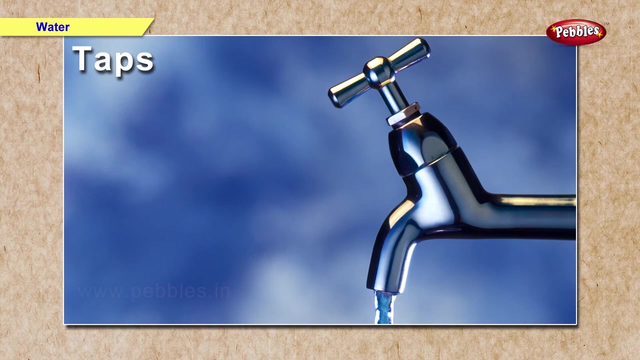 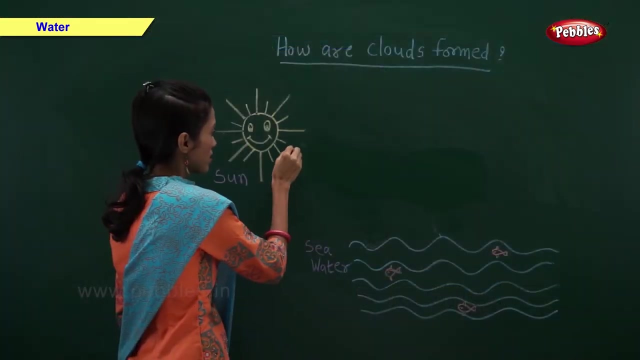 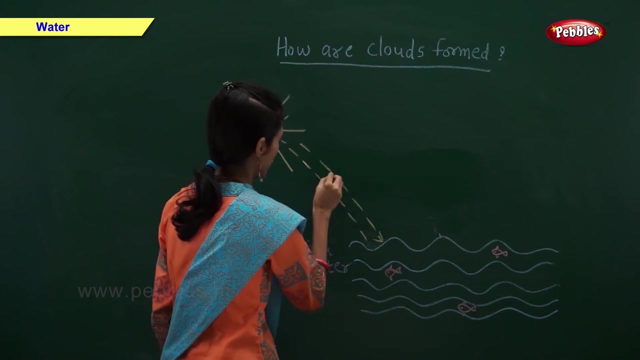 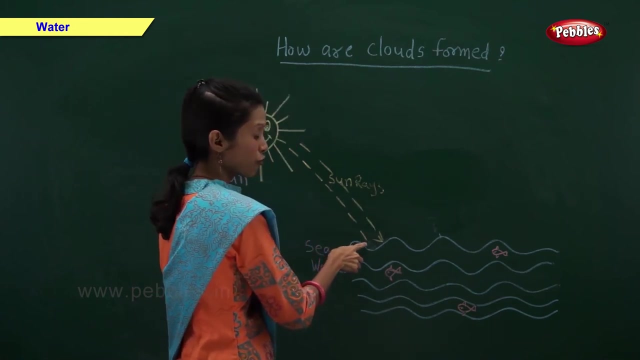 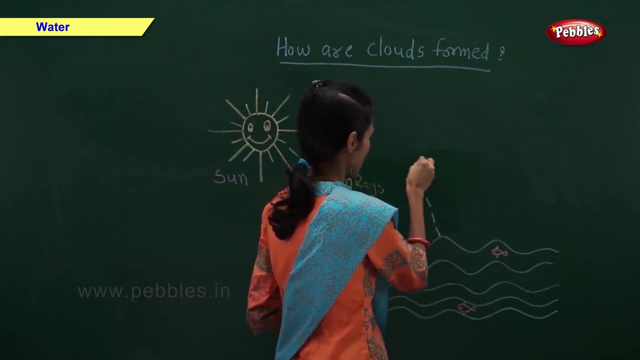 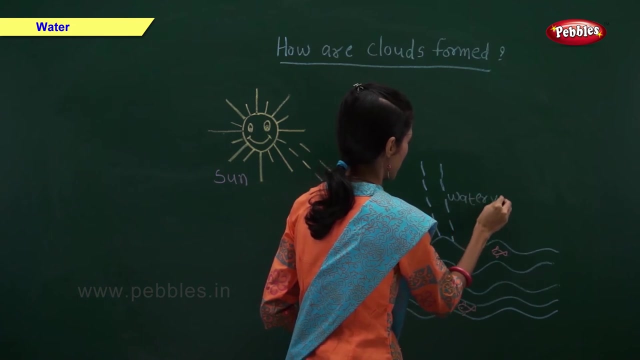 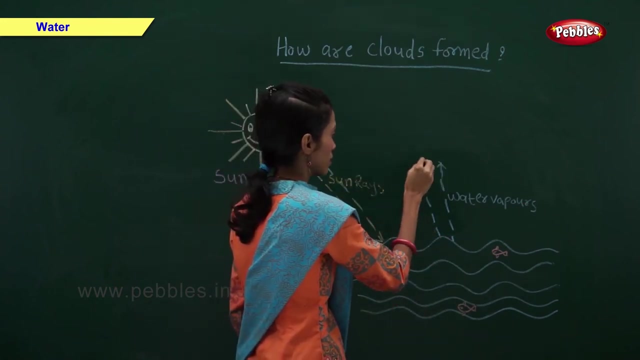 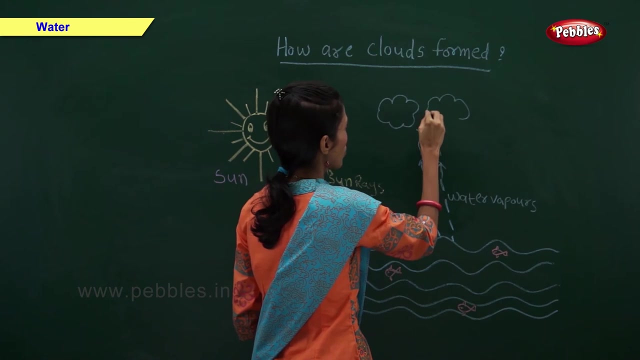 rain sea: rivers, lakes, wells, ponds and taps. Now I will show you pictures of various sources of water. Sources of water rain, Sources of water rain sea. I will show you pictures of water vapours. Water vapours go up and forms clouds. Now let us revise it. 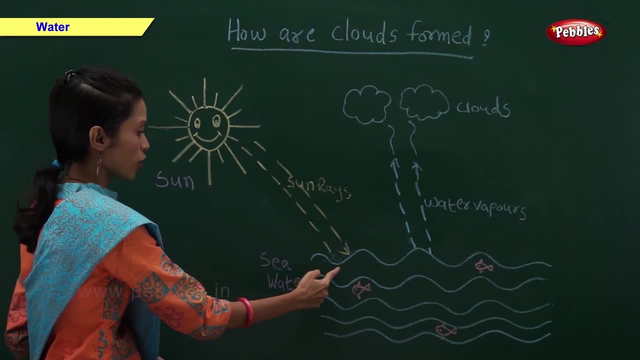 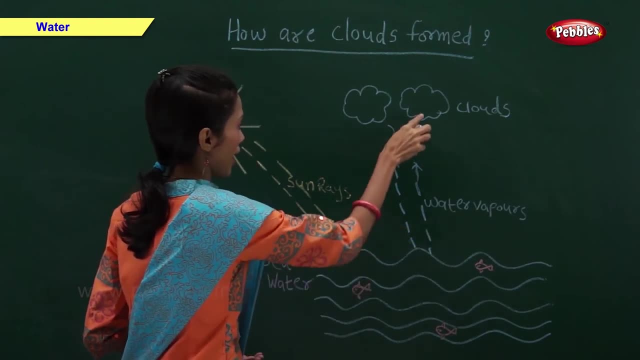 When sun rays fall on a water, water gets vaporized. Water vapours go up and forms clouds. Now let us revise it. When sun rays fall on a water, water gets vaporized. All other laser light stations go up and form clouds. 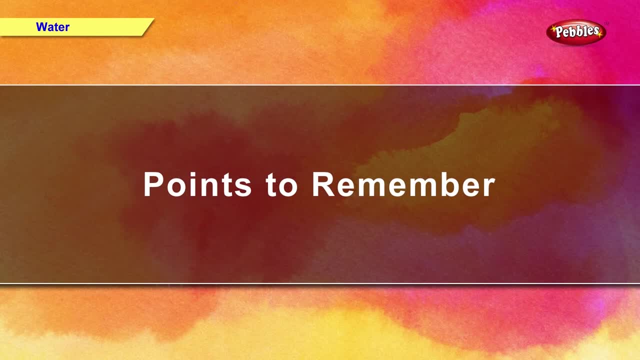 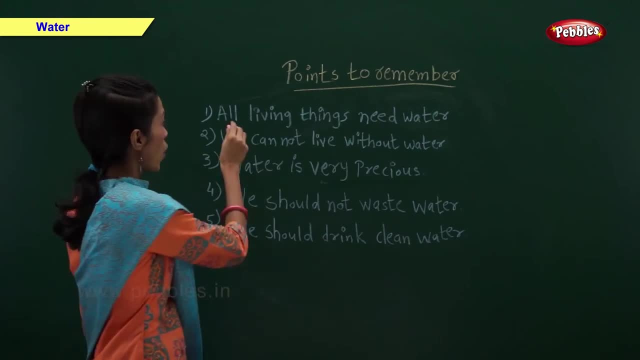 All otherρεアーバー. All other laser light stations go up and form clouds. When sun rays fall on a water, water forms clouds. All other laser light stations go up and form clouds. Points to remember. All living things need water. 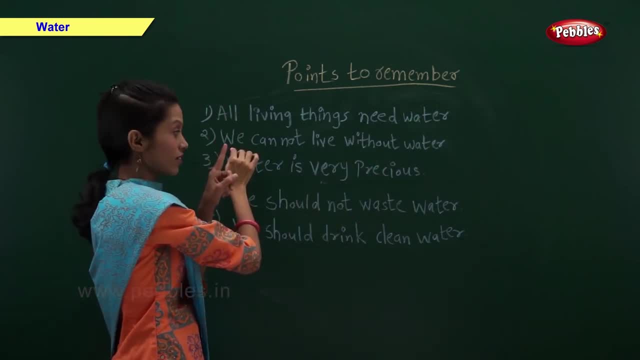 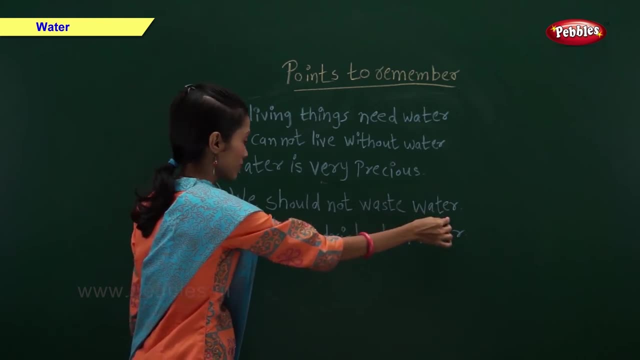 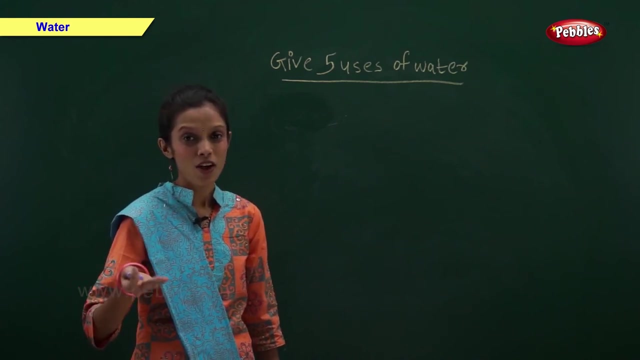 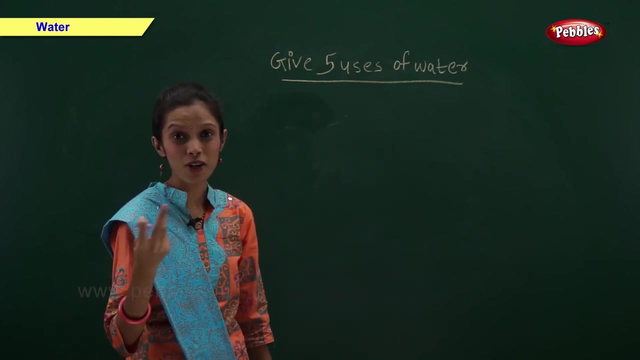 We cannot live without water. Water is very precious. We should not waste water. We should drink clean water. So, friends, now it is quiz time. Now you have to give me 5 uses of water. So tell me fast which are the 5 uses of water. 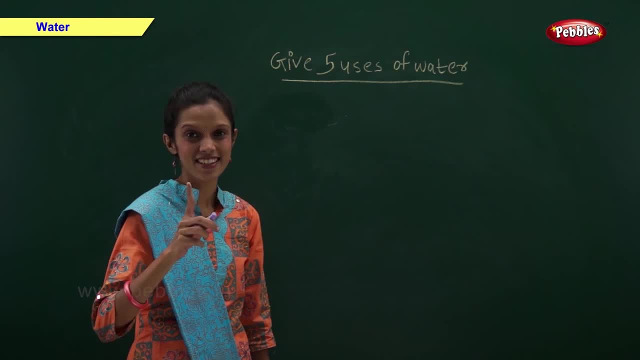 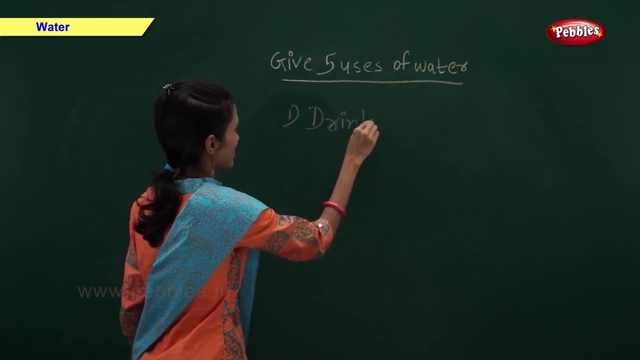 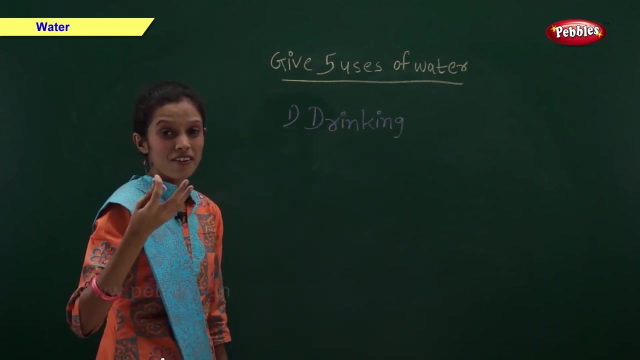 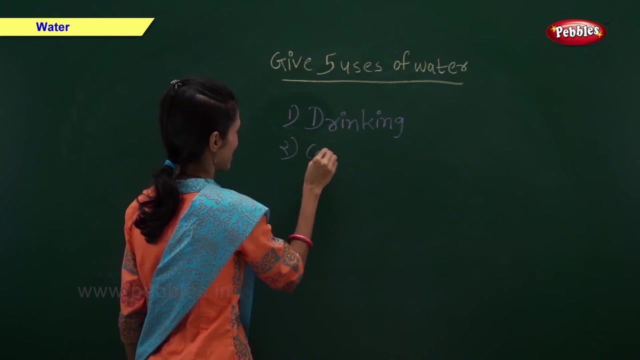 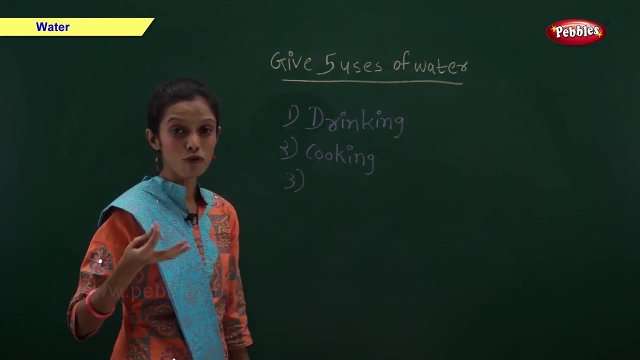 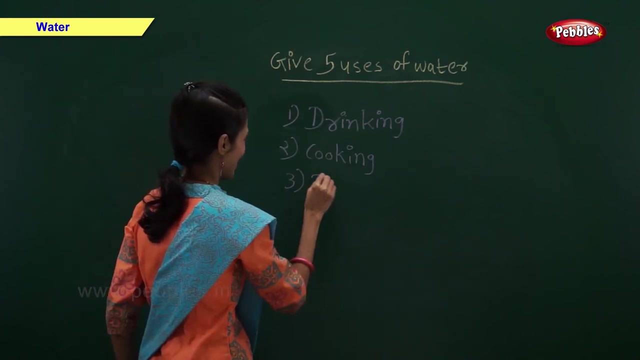 Do you remember I have told you earlier: Yes, drinking. What is the other use of water? Tell me fast. Remember, Yes, cooking. Tell me the other use of water. Remember, Yes, bathing. Tell me other use of water. 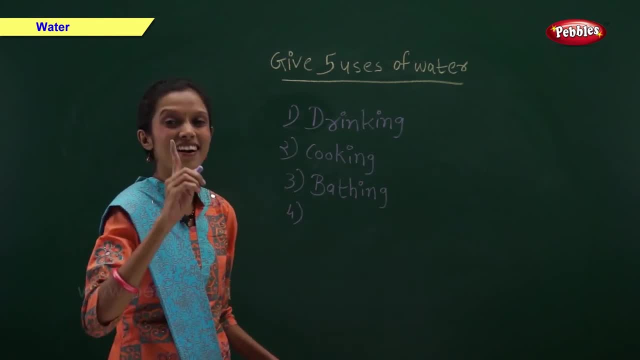 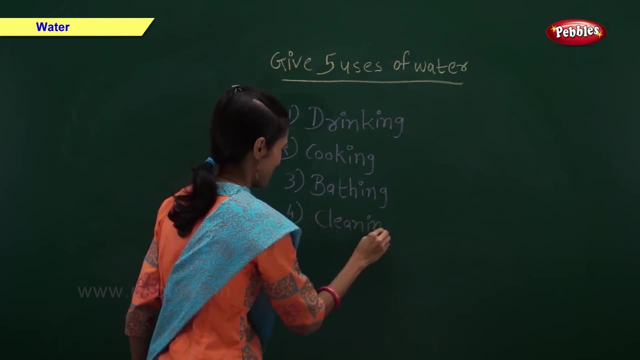 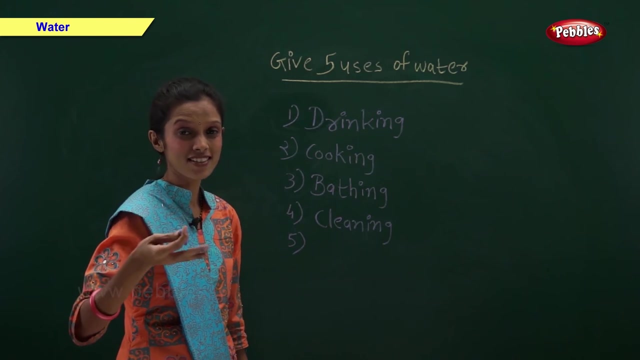 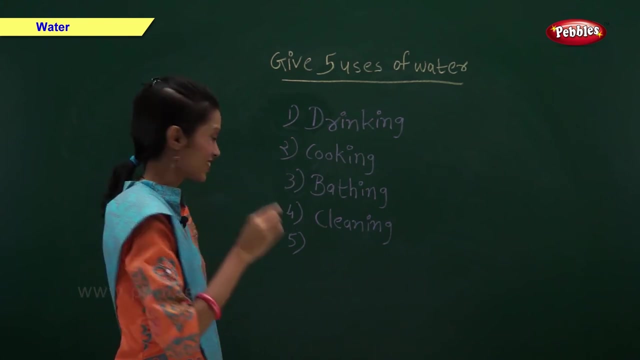 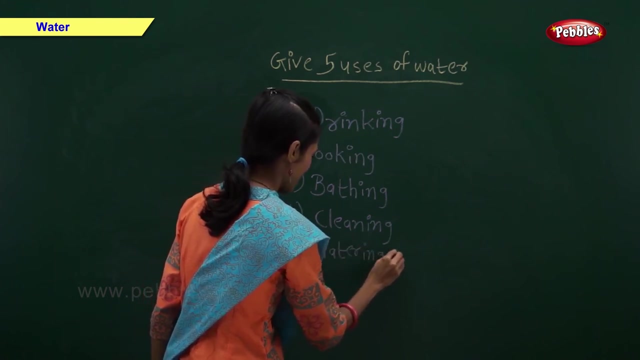 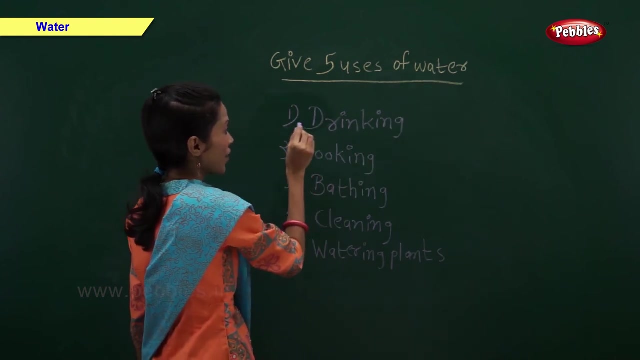 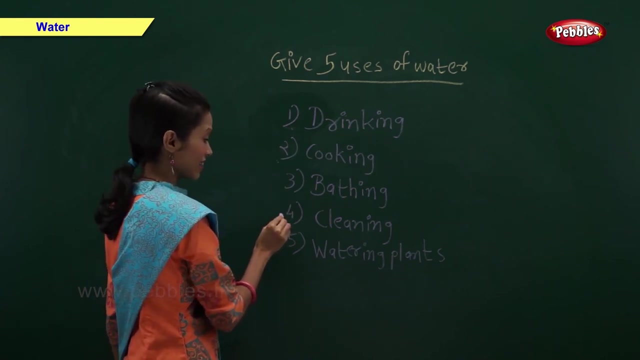 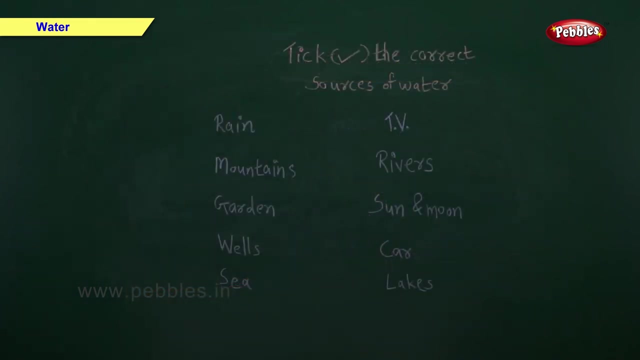 Remember Correct cleaning. One more use of water, Yes, come on fast. Remember, Yes, watering the plants. Yes, water. so 5 uses of water are: drinking, cooking, bathing, cleaning and watering plants. Take the correct sources of water. 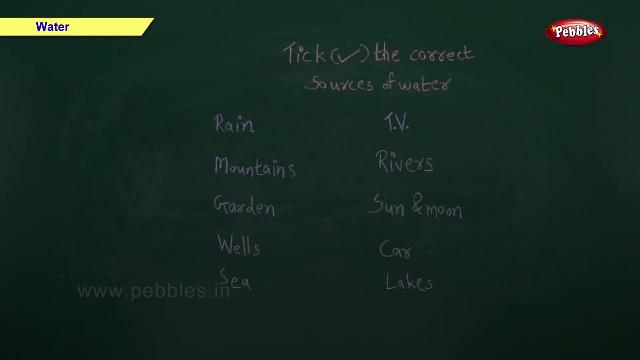 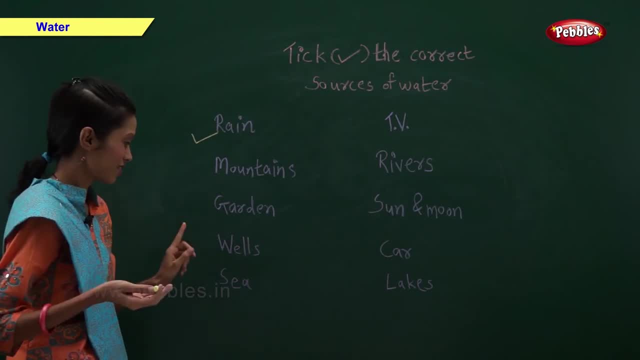 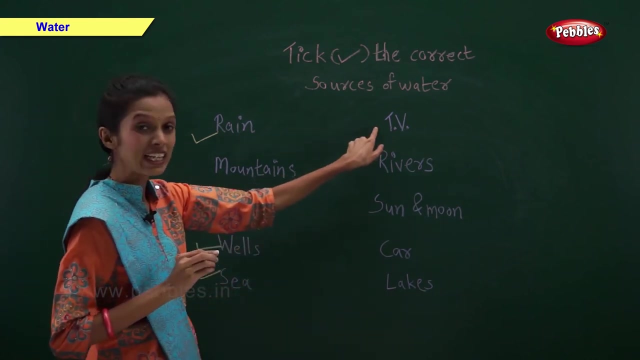 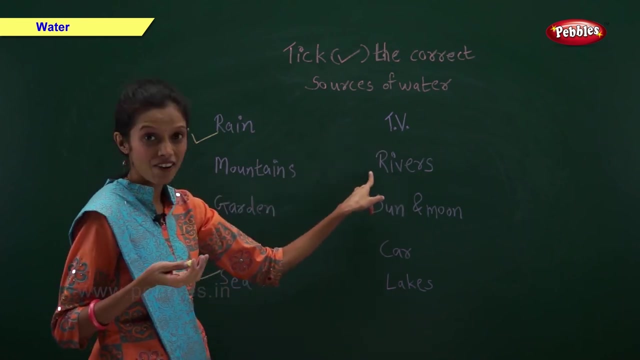 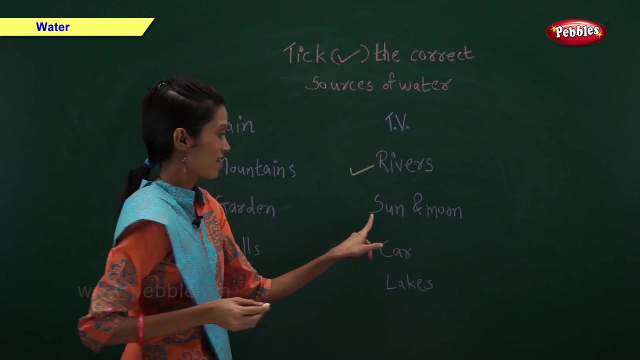 of water? no, it is not. wells are well source of water? yes, they are sources of water. see is the source of water. come on, tell me, yes, you are correct. see is also source of water. TV. is TV source of water? no, it is not. our river sources of water? yes, they are source of water. is Sun and Moon source.